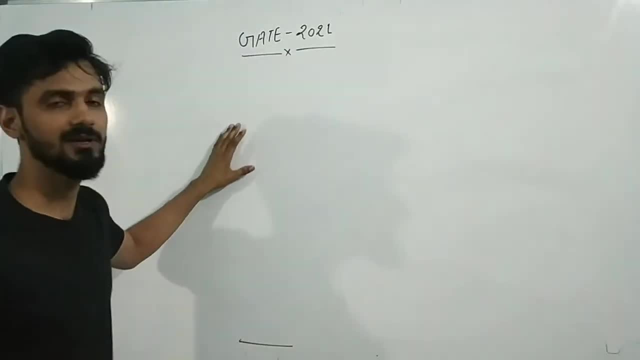 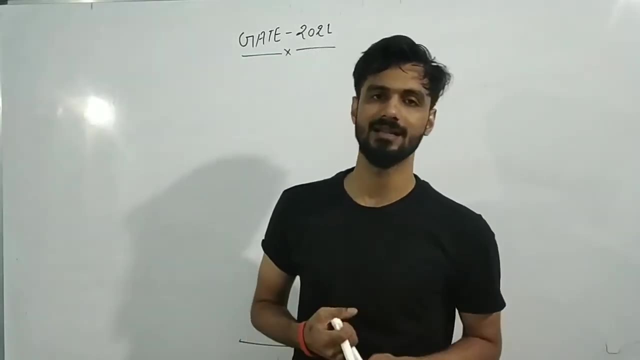 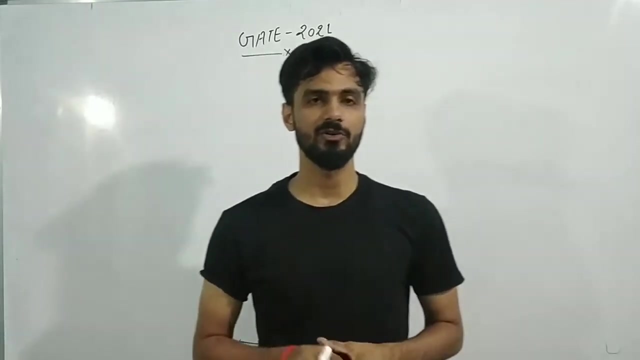 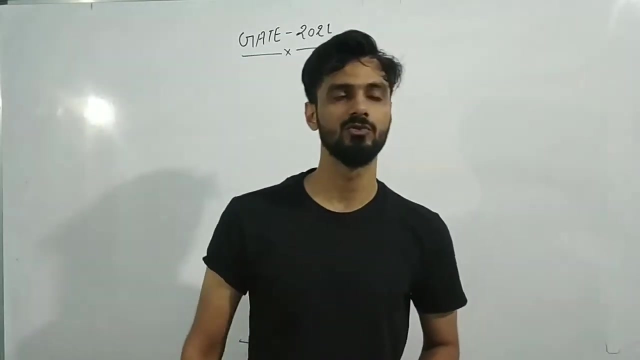 My dear student, I am going to teach you about the next topic in profitability, that is, annual cost. Already I have discussed about the methods from which we can calculate the profitability, just like rate of return, payback period, all these things. Now I am going to discuss about the annual cost. It is also one of the important methods to calculate the profitability. If you are going to compare two assets, which is more attractive for the investment purpose, then this is one of the most important methods. 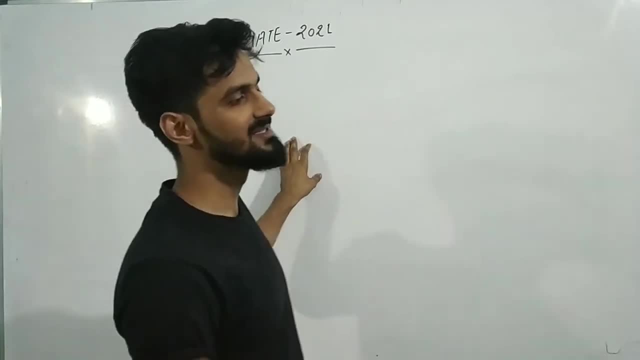 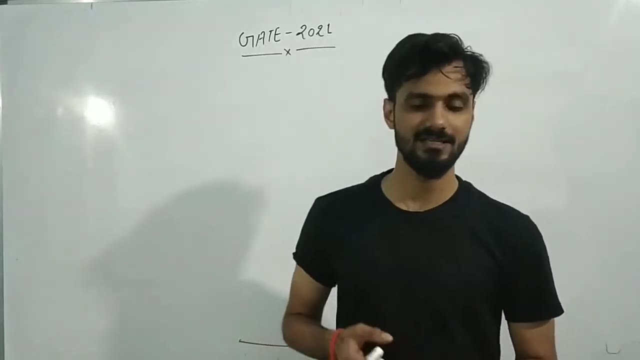 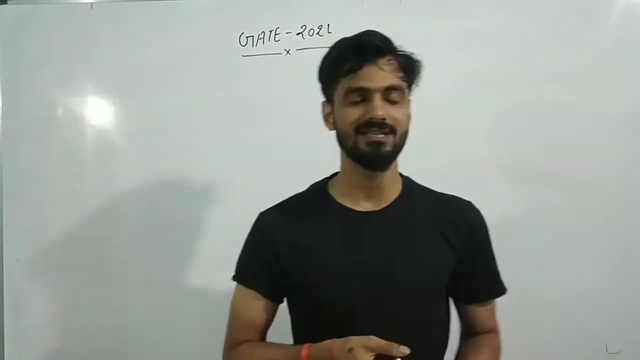 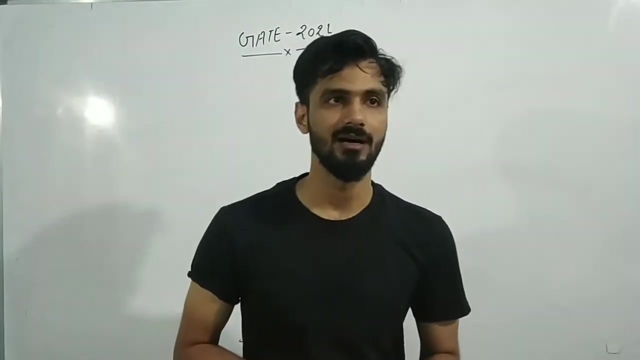 This is a method that you can use Now, if you will see where we can use this method. So just understand if the service life of two assets or two capital is going to be different means just like understand one thing: if you are assuming a capital or an asset A having a service life is 10 years and an asset B having a service life of 15 years, then it would be inappropriate to calculate the, you know to compare the assets or where you want to going to invest the capital or where you want to invest the capital. 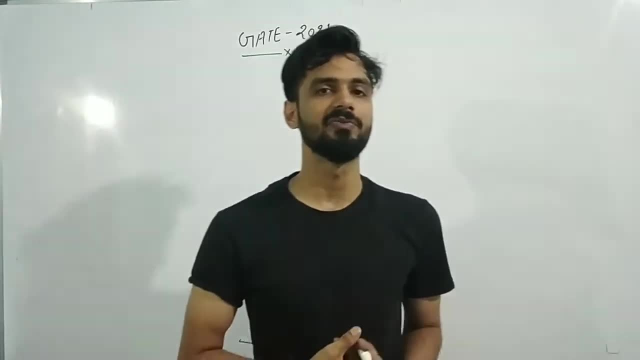 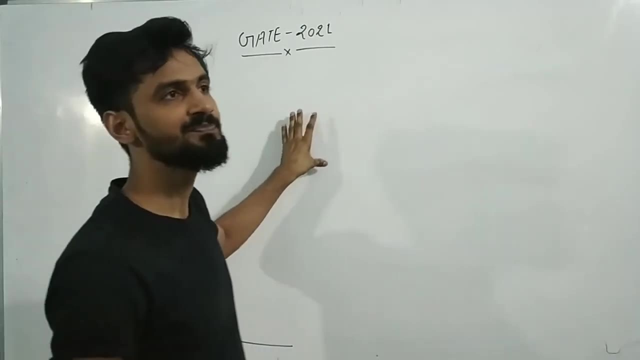 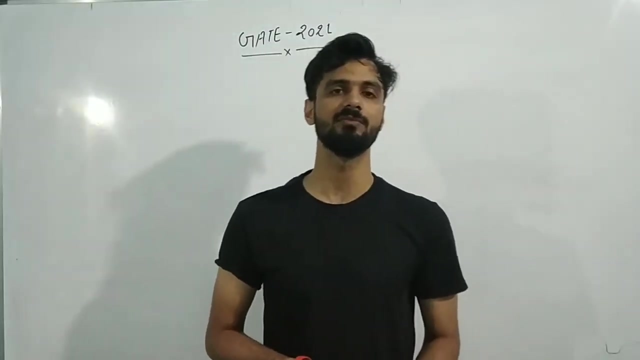 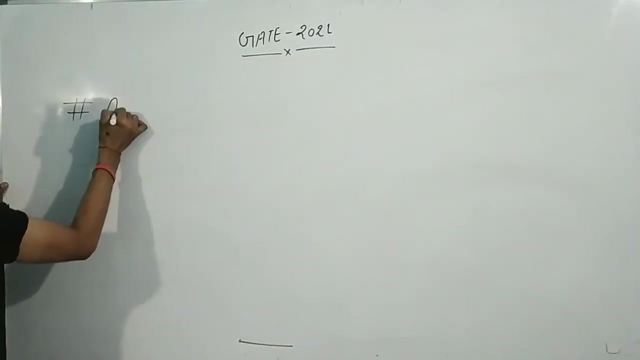 On the basis of net present value. So it would be inappropriate for that. So to avoid this mistake, we will use the annual cost method for the selection of our capital, for the selection of our project, so that we can invest the amount of money on that particular project. So if you want to define the annual cost, I am writing the definition So you can define annual cost. 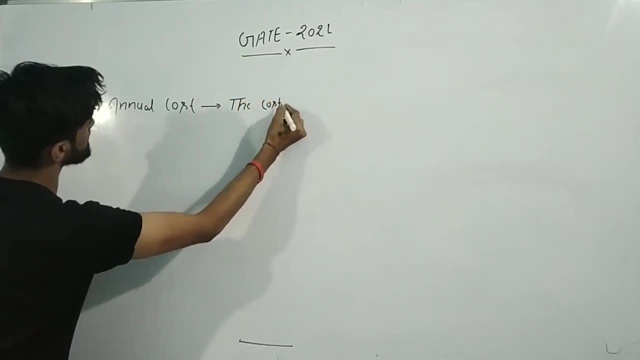 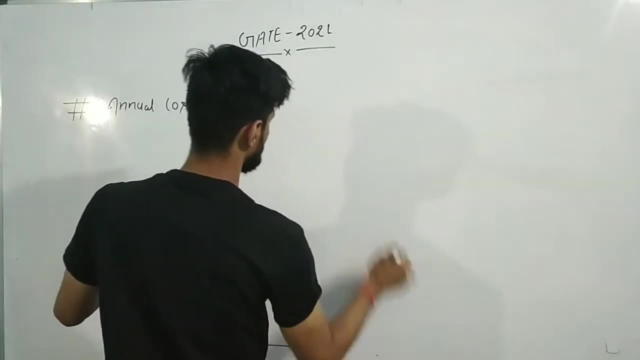 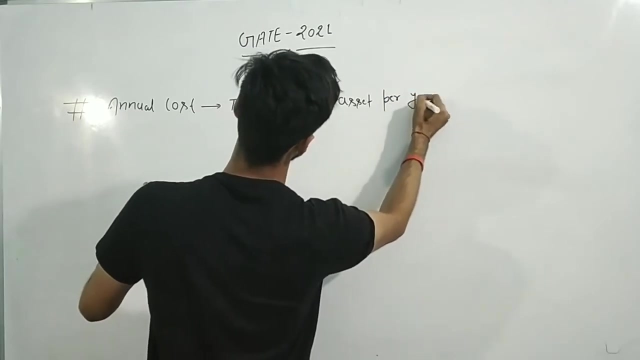 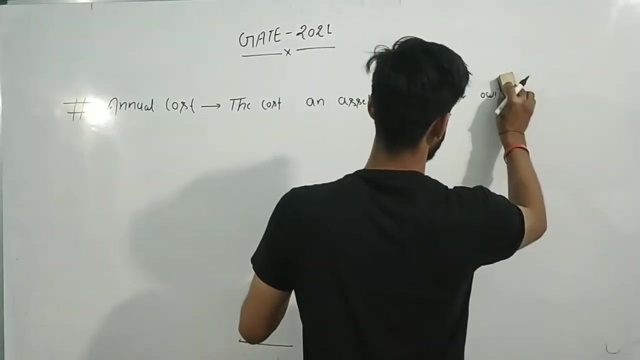 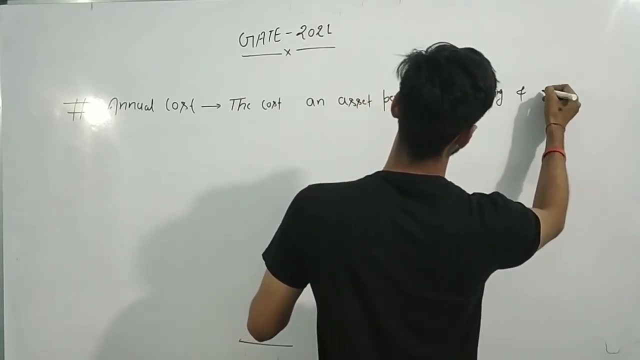 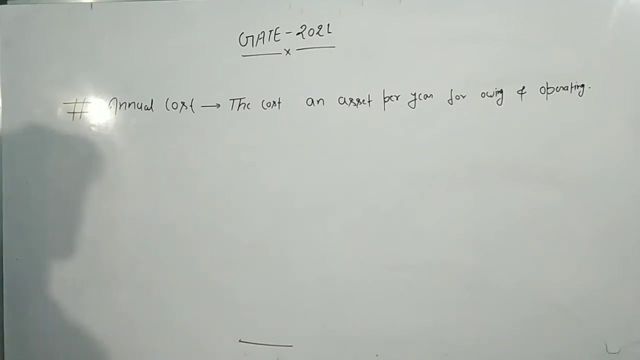 The cost, the cost of the cost of an asset per year for owing and owner operation. the cost of an asset of an operating per year is called the annual annual cost. now already I have told you you will assume I am just assuming asset A and asset B. 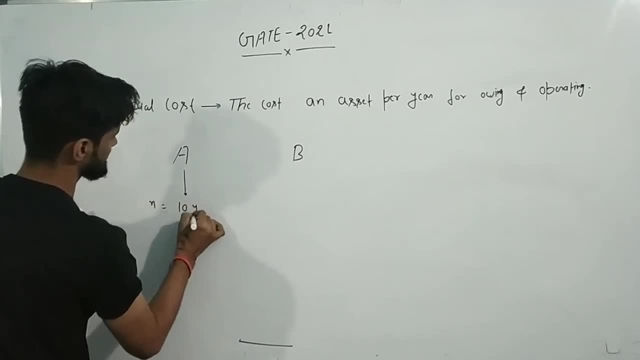 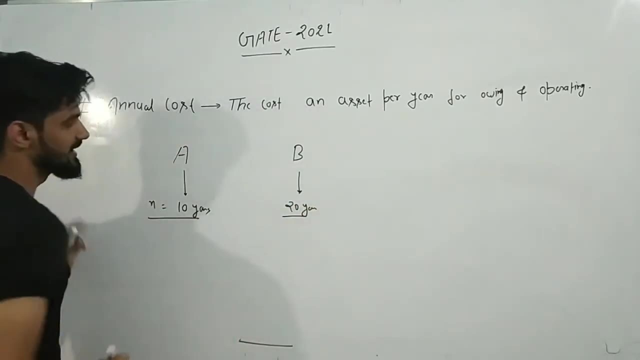 having its service life is equal to 10 years and having its service life is equal to 20 years. ok, now it would be inappropriate to judge the project where we can invest the money and which project will be more attractive according to the basis of net present worth. 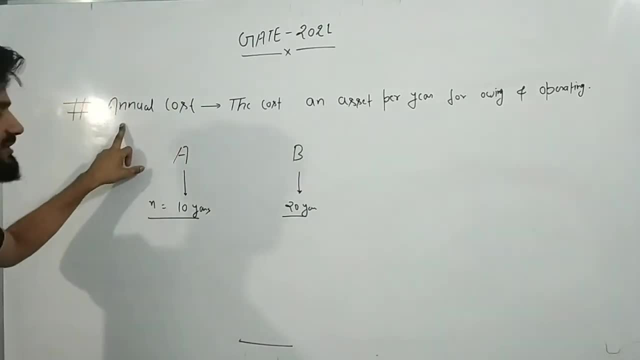 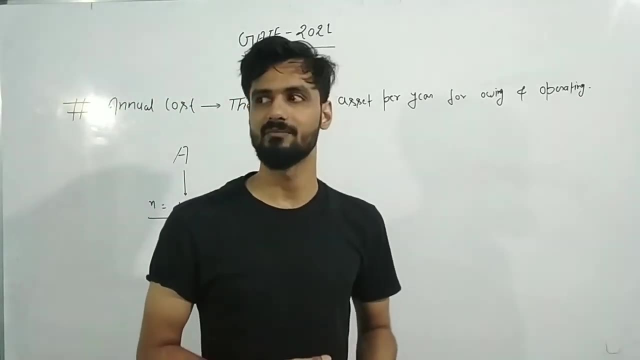 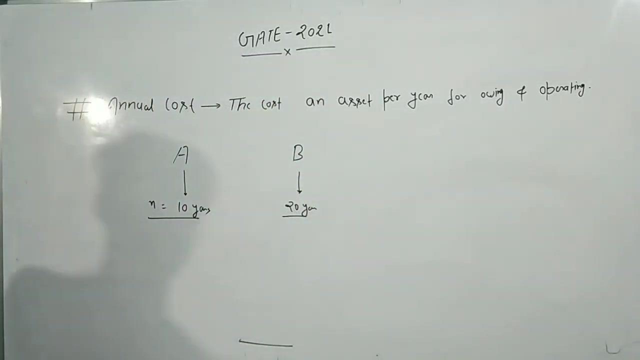 so, to avoid this mistake, we go to calculate the annual cost method and the object or the asset having less annual cost that will be more attractive as compared to the asset having more annual cost. ok, so on that basis we will be calculating this thing. now understand one thing. 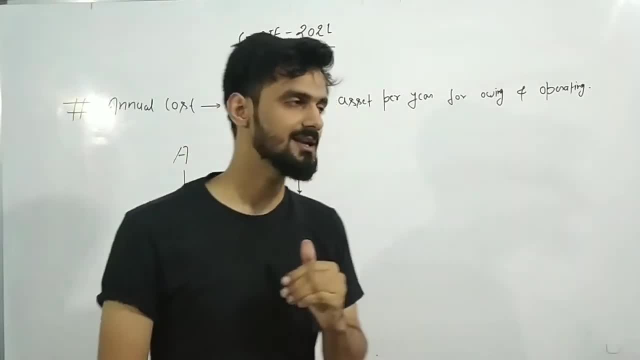 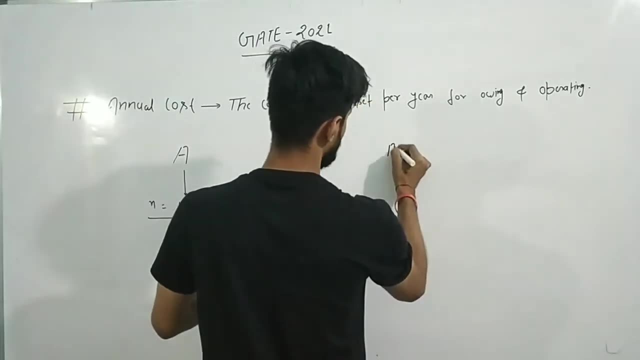 in annual cost method what we use to do generally. I am taking you, I am letting you to understand, with the help of an example, if you will feel, if you will understand, if there is an asset, A ok now having service life. N is equal to 10 years. 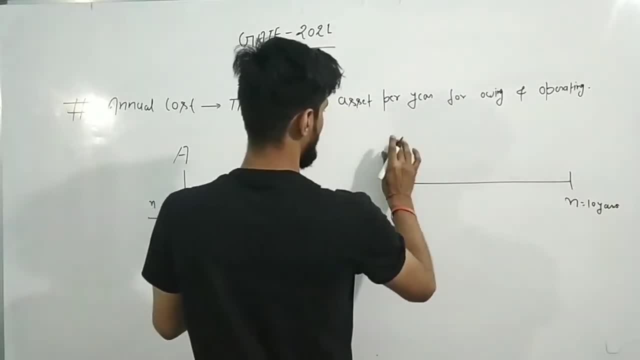 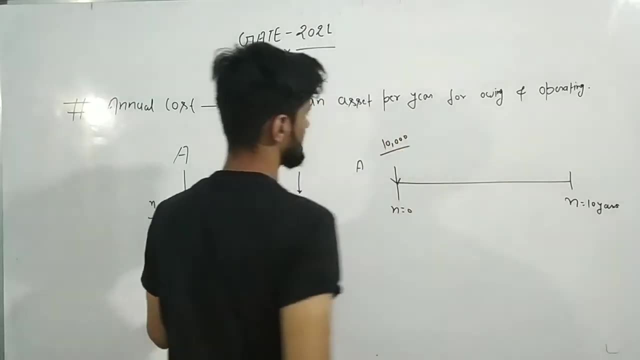 understand. having service life is equal to annual 10 years. and now for A you are just placing at N is equal to 0, an amount of 10,000 of rupees. now what will happen? you have to calculate this 10,000 rupees. 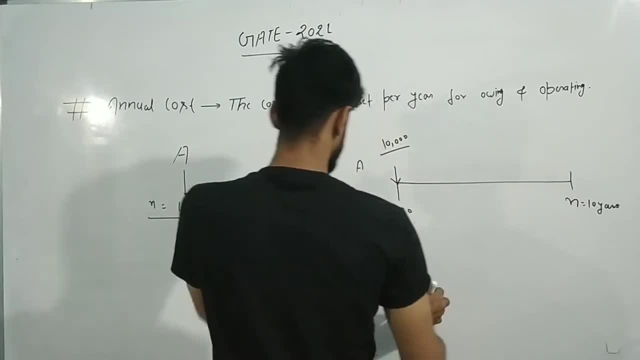 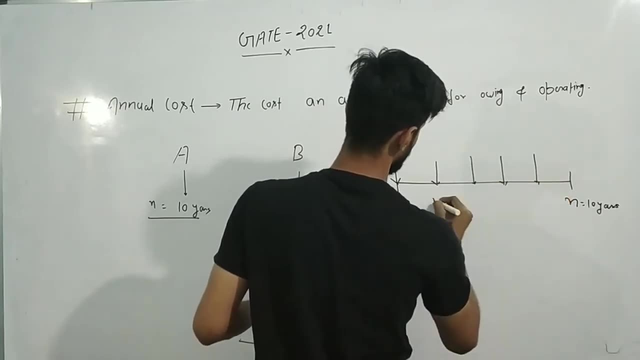 in an annual way. so if you want to calculate this in an annualized cost, then what will you do? there will be some cash inflow every year. at N is equal to 1, at N is equal to 2, at N is equal to 3. 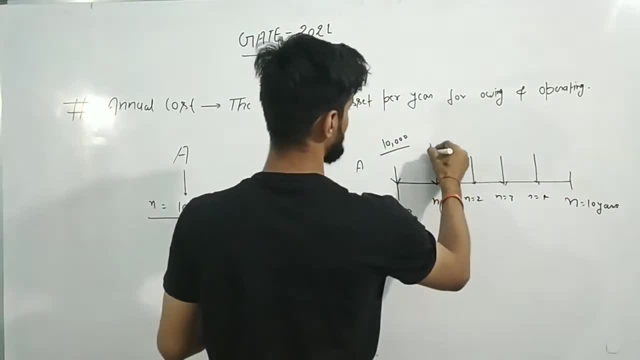 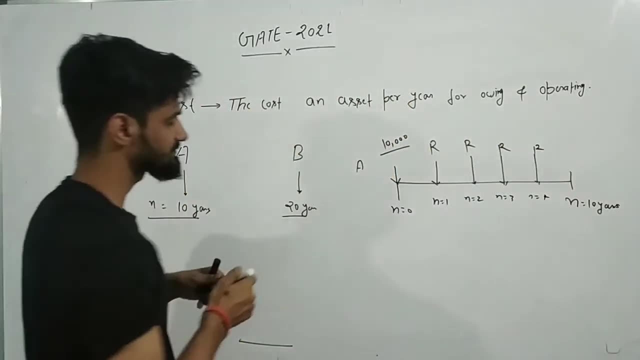 at N is equal to 4. ok, just like, if you are getting annual cash flow of R R every year up to 10 years, then if you will think here, then what will happen if you are going to convert all this R value of R in the present value at N is equal to 0? 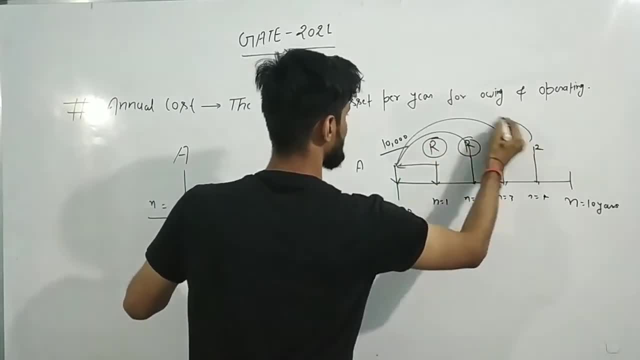 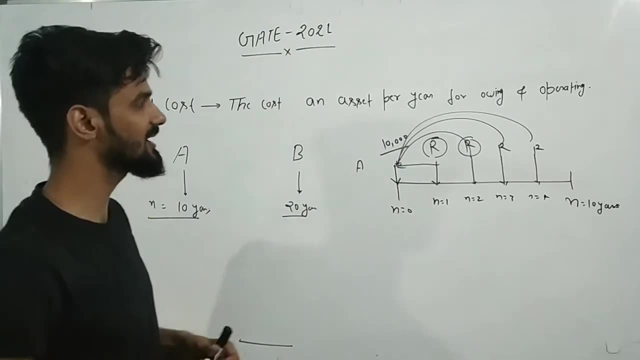 at N is equal to 0, then what will happen after converting all the cash flow? all the cash flow in its present value? and if you are going to add the present value of all the cash flow at N is equal to 0, then you will be getting the original amount of money. 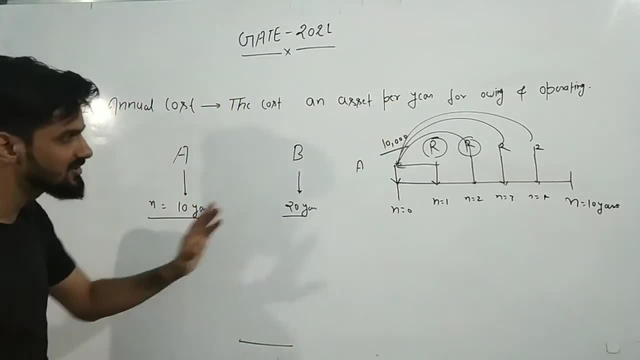 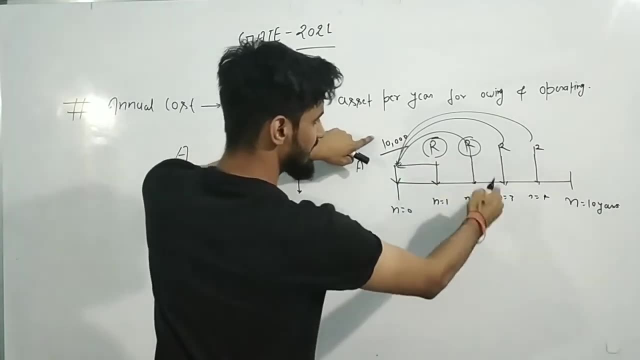 that you are going to invest for a particular asset, A. so just write down the question: how will we convert? so, if you will see then how this 10,000 rupees get equalized, get distributed in a series of payment, you will see in a line source method. 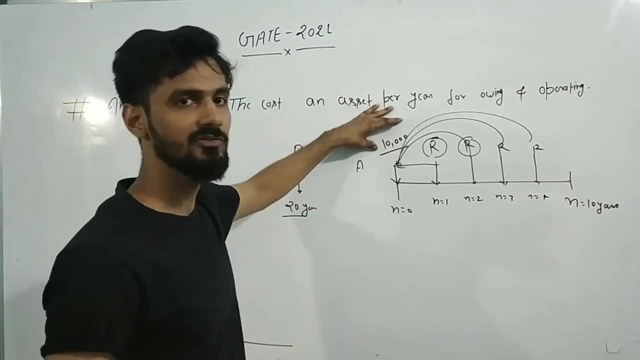 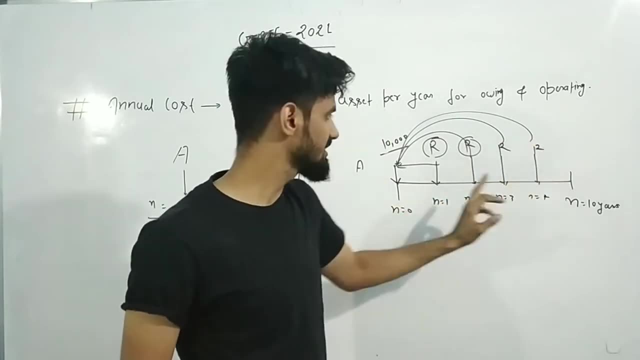 a particular amount, an original amount. the original amount of an asset is going to be, you know, cash flow, in the form of in cash flow in a series of payment. ok, here you will see there is: a value of R at N is equal to 1. value of R at N is equal to 2. 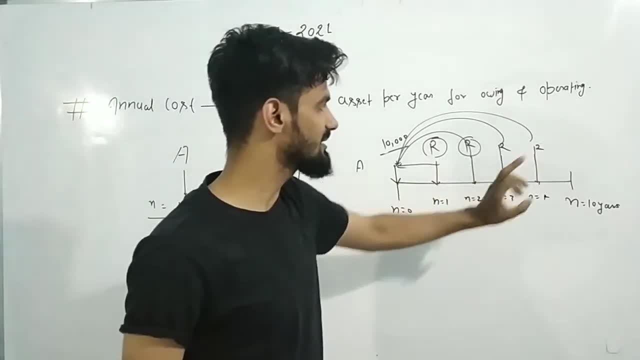 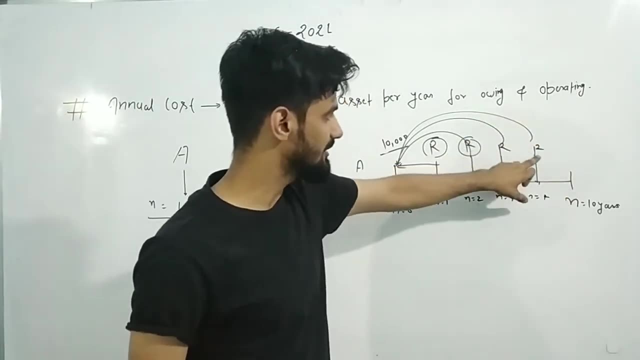 value of R at N is equal to 3, you are getting the value of R amount that is, a series of payment in a particular year. and if you are going to convert all these- the value of R- in the present value, then after adding all these values, 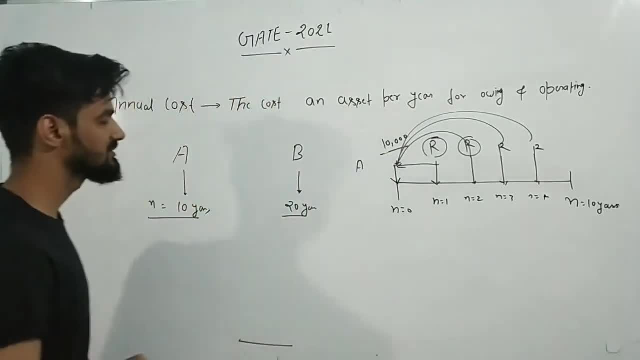 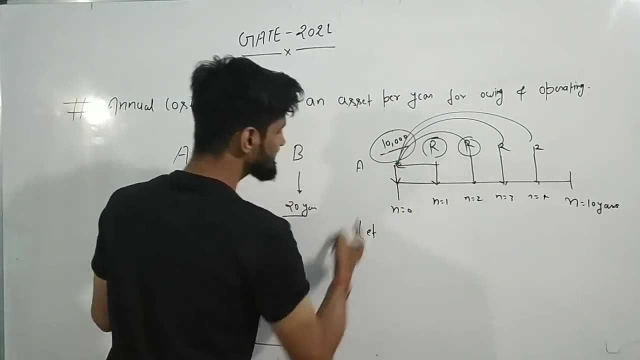 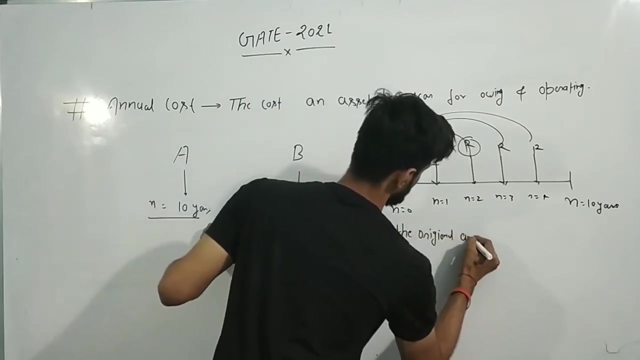 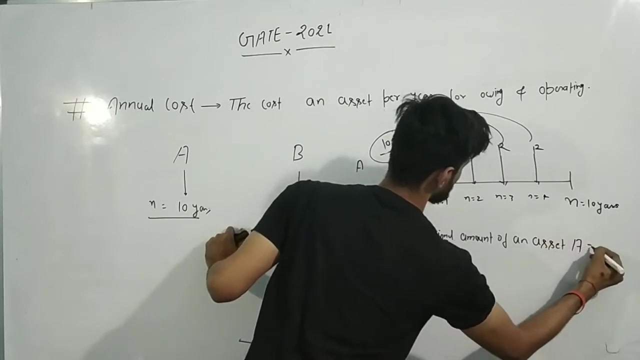 you will be getting the initial amount of that asset. how will we do? just understand one thing. so if you want to calculate, just understand. I am taking, let let's. let's suppose let the original amount of an asset A is equal to P. I am assuming the original amount of asset A is equal to P. 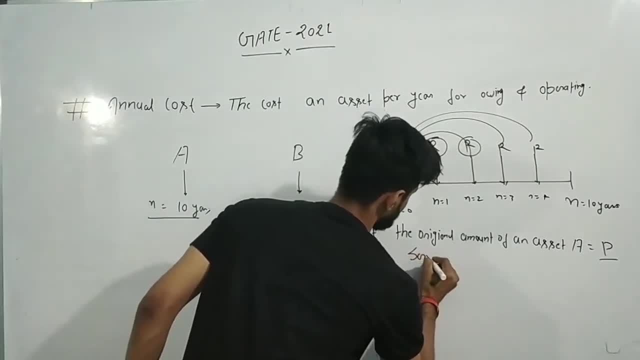 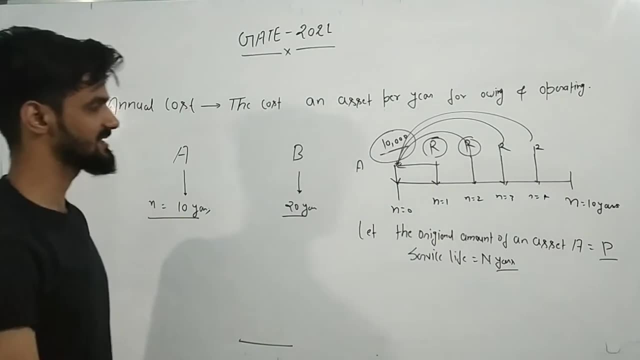 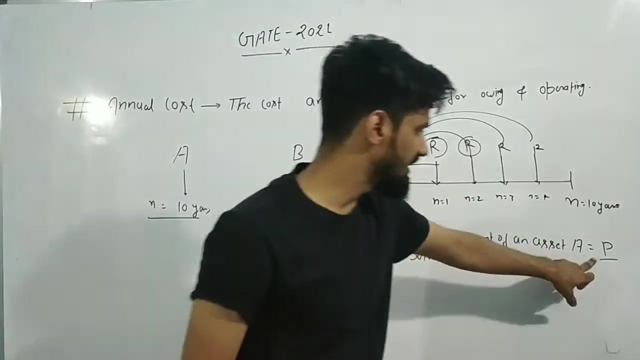 now the service life of an service life. I am writing service life that is equal to N years. service life of this asset is N years. now, if you want to calculate the annual cost of this particular original amount throughout the whole N life service for the service life of N years. 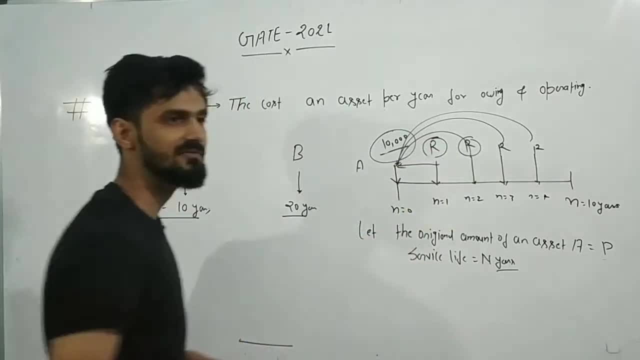 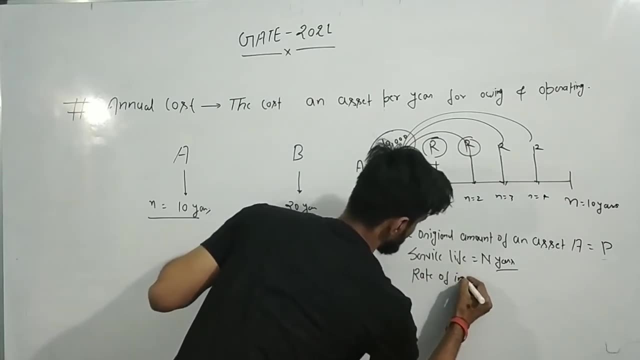 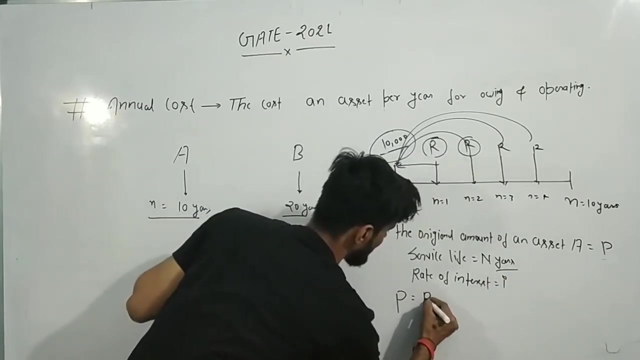 then you can calculate with the help of a formula and it will follow the concept of annuity. it will follow the concept of annuity and if rate of interest that is equal to I, then you can calculate P is equal to R into 1 plus I to the power N. 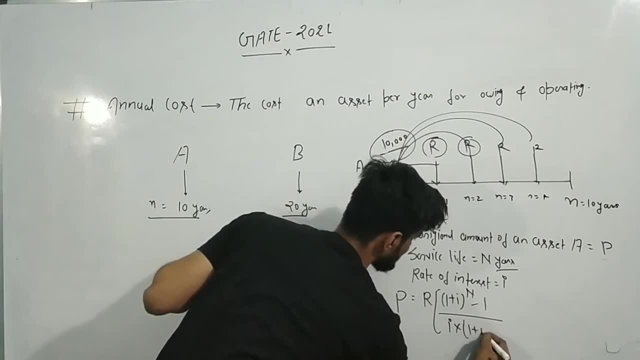 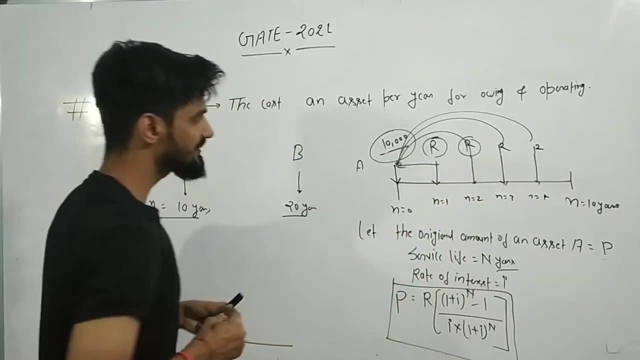 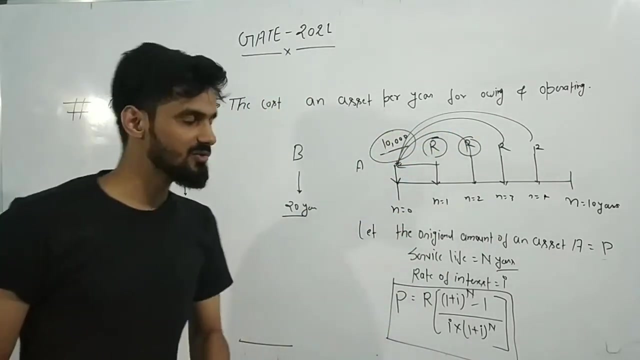 minus 1 upon I, multiplied with 1 plus I to the power N. this is one of the important formula because it will follow the concept of annuity, because each and every year you are getting some cash flow to the project and generally what you are doing right now. 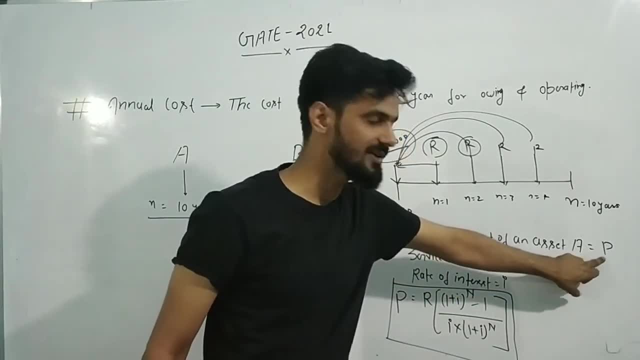 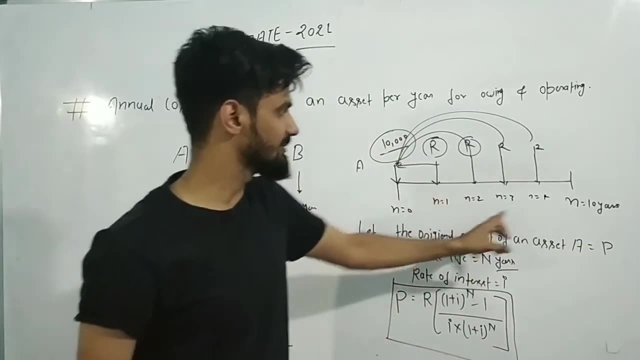 you are doing, only you are just getting, you are just converting this value of P in annual cost each and every year, how much amount of money that you have to invest for this for throughout the whole service life of N years for a particular asset. so if you will see, 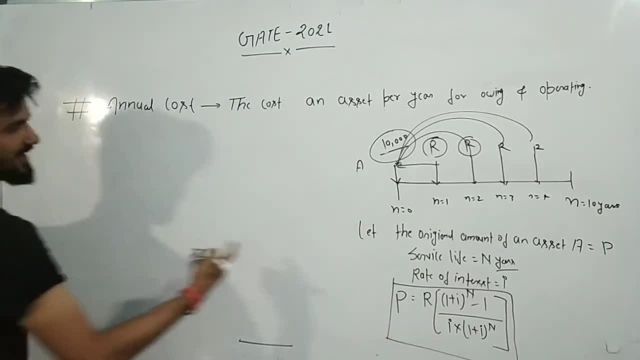 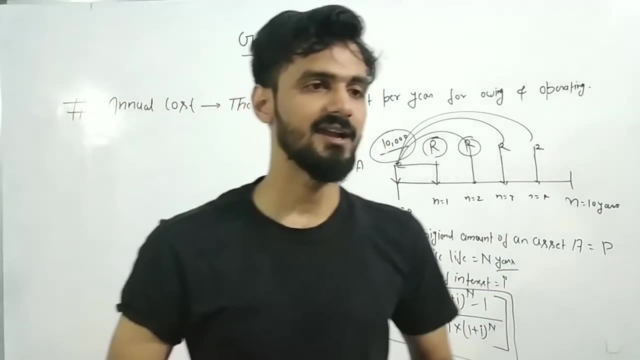 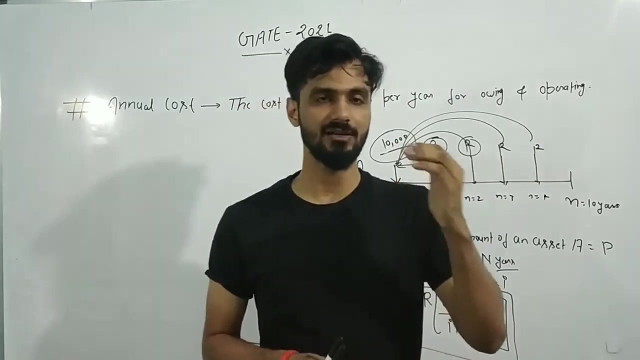 then I am writing here: P is already I have written, P is the already I have written. P is the original amount of the assets and N is service life of an asset and R is the annual cash flow. annual cash flow, you can assume it the annual cost for that particular asset. 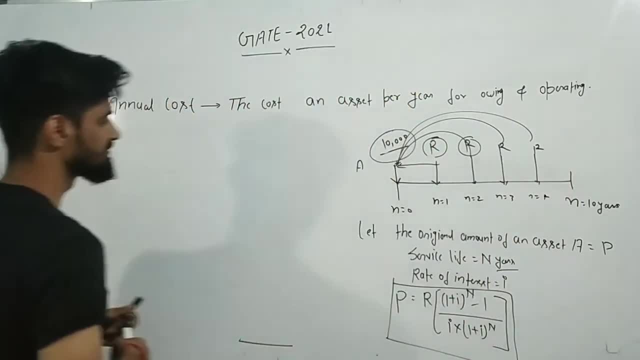 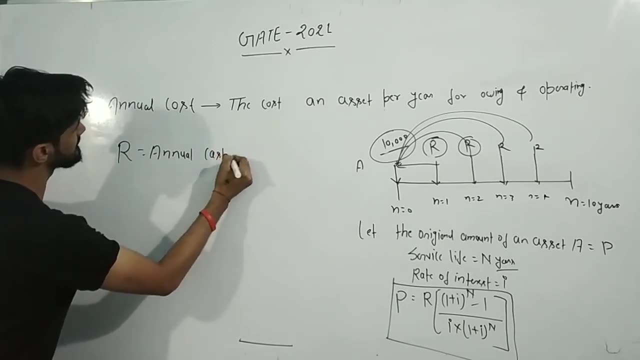 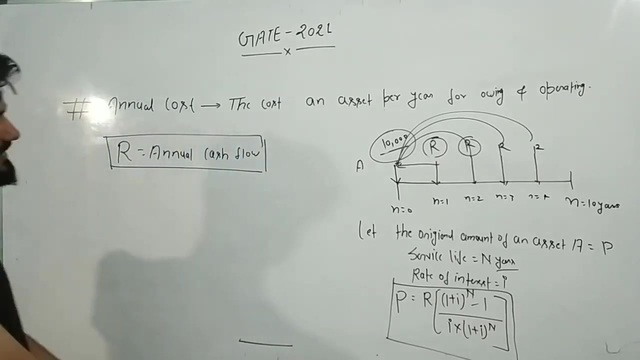 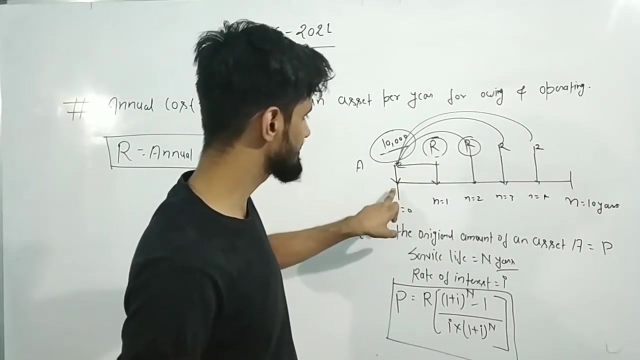 that is getting inflow for the project. so here I am writing: R is annual annual cash flow. here, R will be annual cash flow, my investment. and there is one thing: what used to happen here? just what I am telling you is very simple thing: if you will convert this R into its present value, 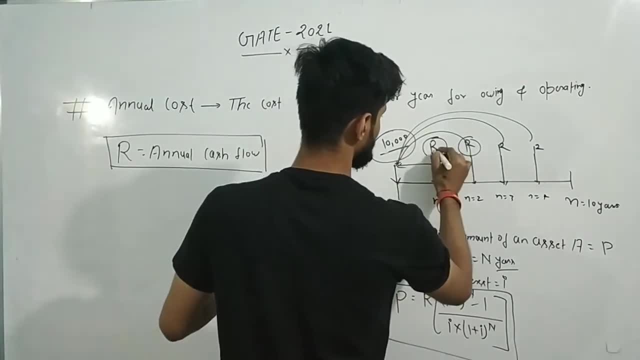 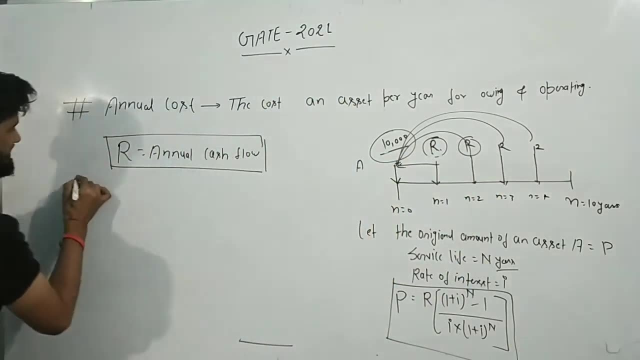 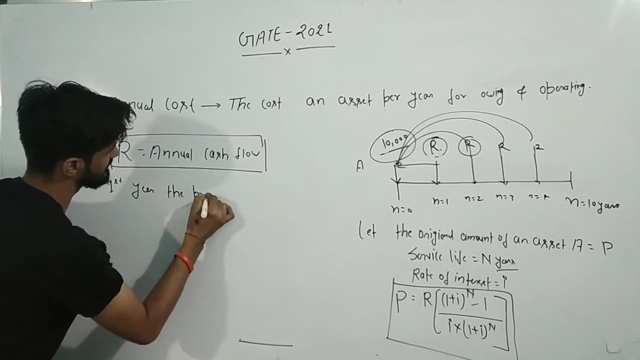 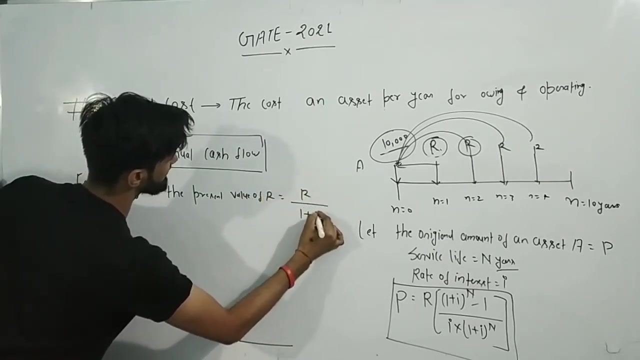 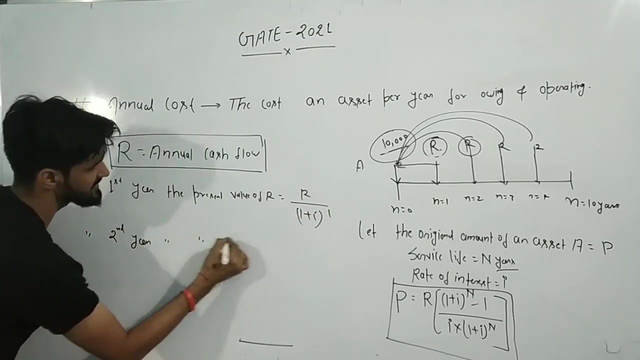 then how will you convert? just, I am writing here: this is R, this is R, this is a. so I am just trying to convert this R into its present value. so for first year, if you will write, for first year, the present value of to what r upon 1 plus i to the power of 1, for second year, the present value of r Again. 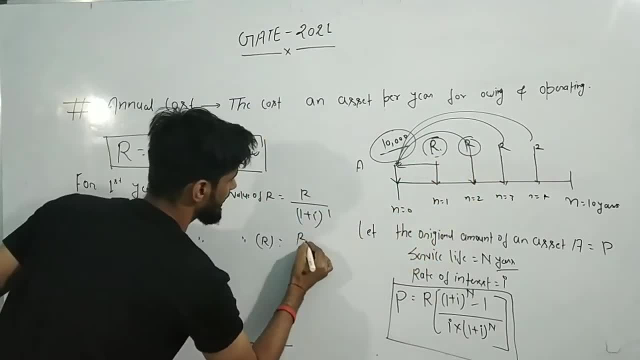 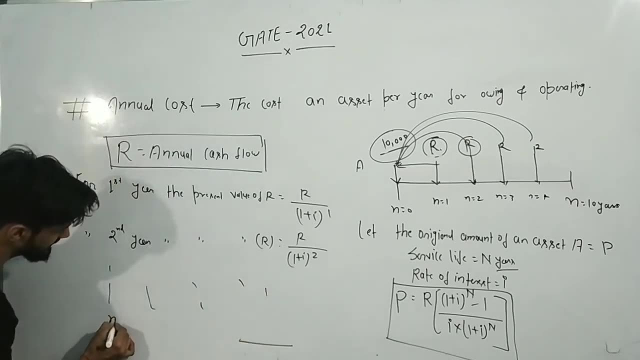 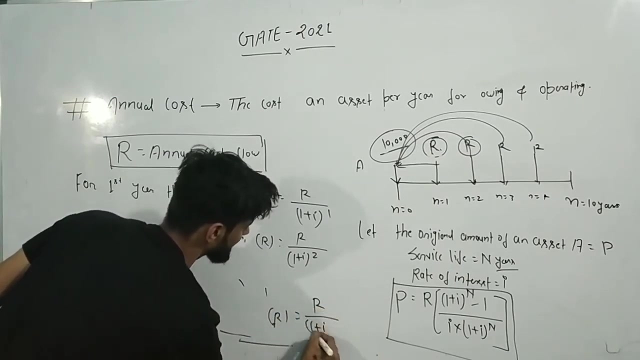 there is a cash flow of r in the project, then that will be equal to r upon 1 plus i to the power of n. So if you are going to calculate for n year, then you will be getting present value of r is equal to r upon 1 plus i to the power of n. Now what I am trying to tell: 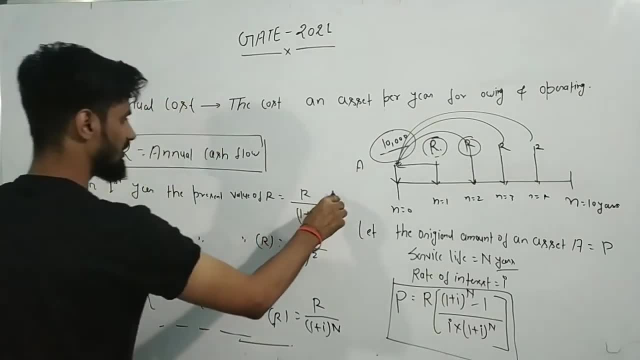 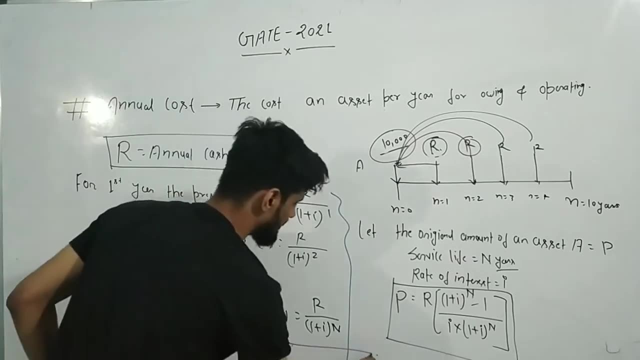 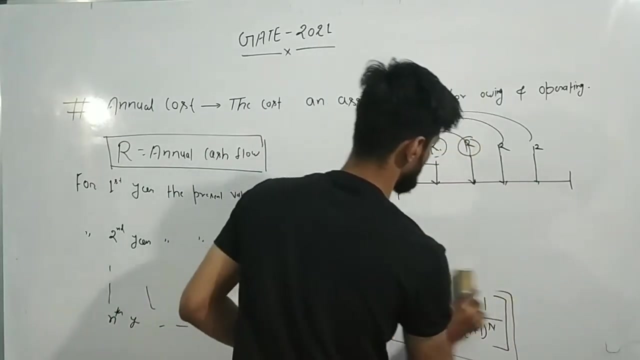 you is a very simple thing. If you are going to add all these things, because already you have converted all this cash flow in its present value. Now, if you will add all these things, then what will you get? I am just dropping it out- Then you will get a value. So you. 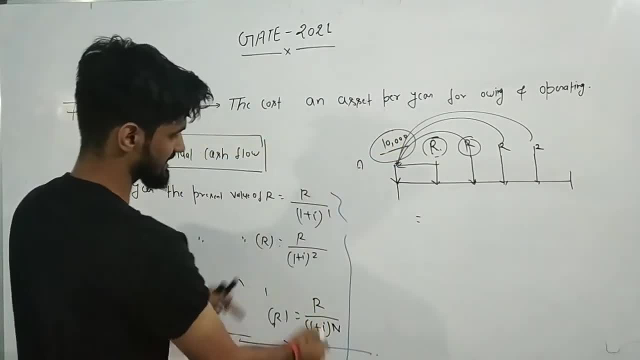 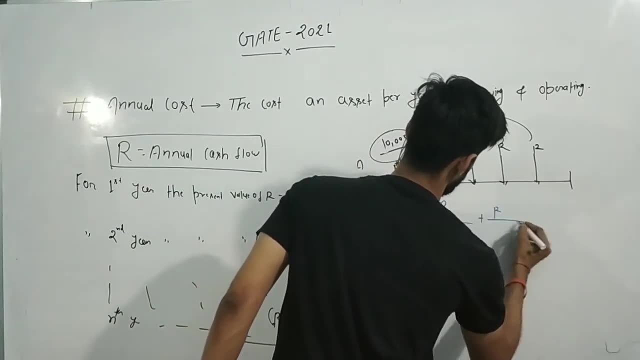 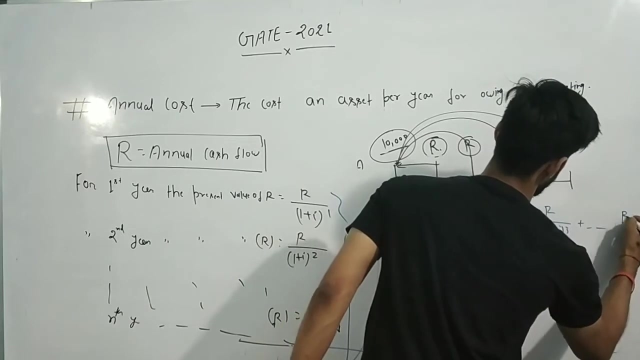 will get a value. I am just going to do the sum of this particular value. I am just going to do this particular thing and summing it out. then you will get r upon 1 plus i, plus r upon 1 plus i to the whole s to y, plus r upon 1 plus i cube, plus dot dot r upon 1 plus. 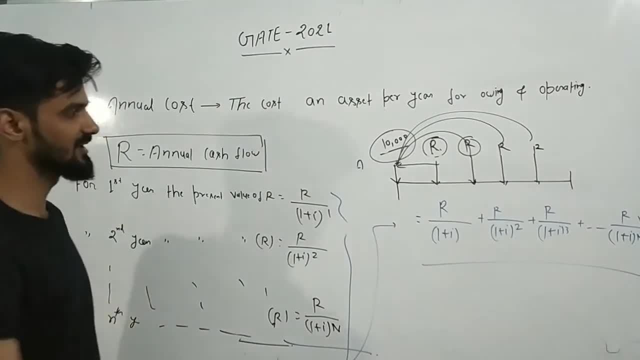 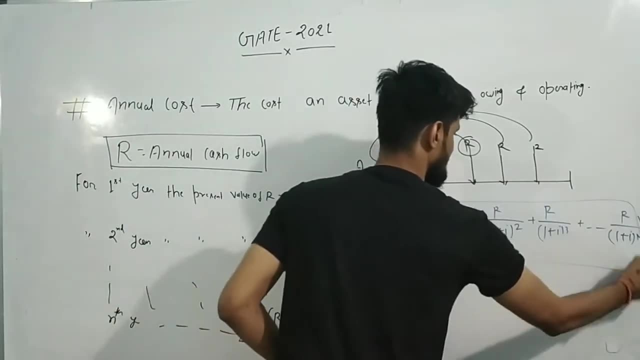 i whole n. So now my idea is that what is this value? This is a term that is a gp, and this will give you the value of present worth. So here what I am trying to do: I am just converting all these things. 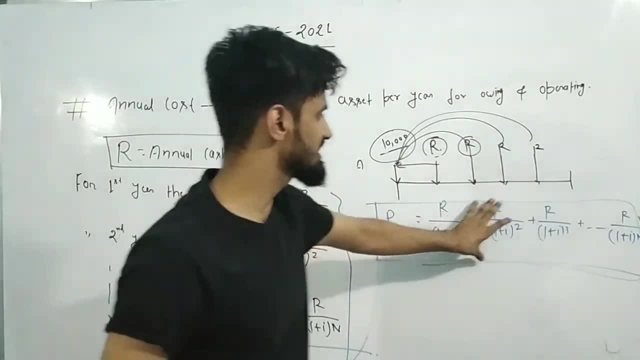 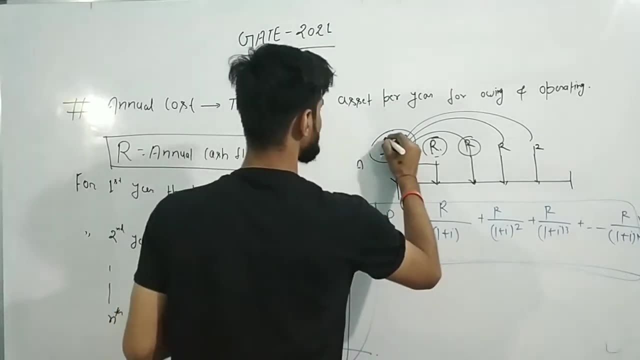 I am just adding all the value of cash flow in its present value and I am just adding all the sum of this present value and it will give you the present value of the asset. So this is the present value of asset A. So if you will calculate, if you will solve this, 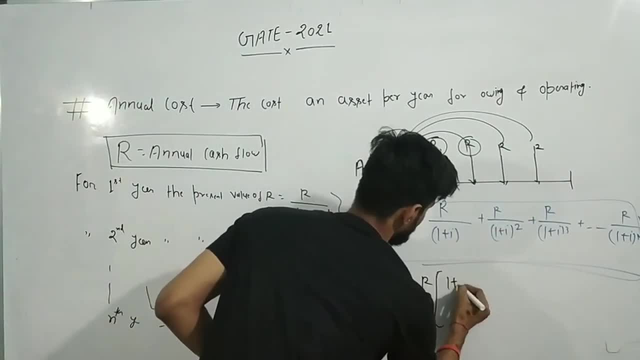 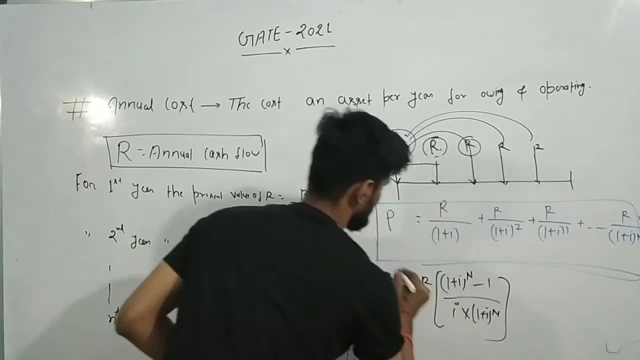 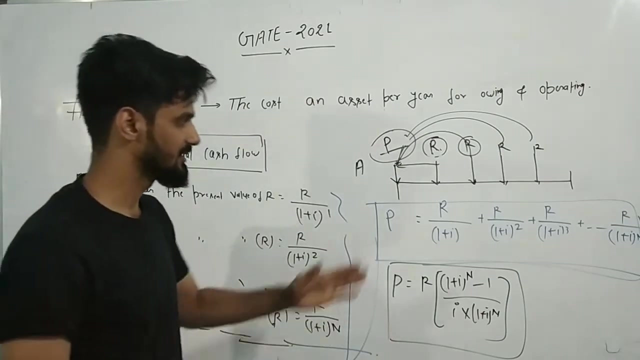 then you will be getting p is equal to r into 1 plus i whole to the power n, minus 1 upon i multiplied with 1 plus i whole to the power n. So this is the derivation part in the annualized cost. So now you understand one thing I will tell you later on with the help of an example. then, 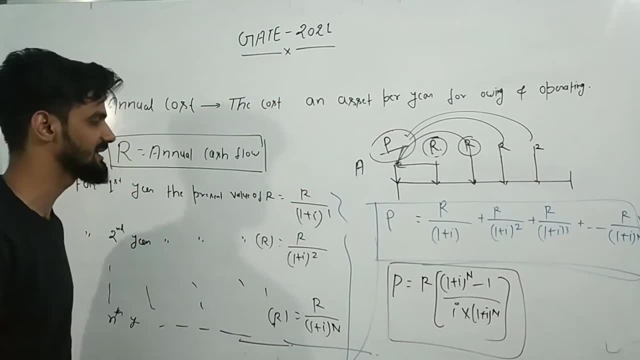 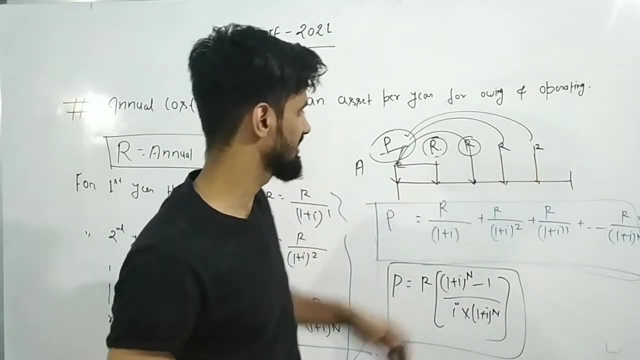 it will be very clear to all of you to understand how you will calculate the annualized cost. I think up to this. it is very easy to calculate annualized cost already. if the cash flow is, you can see: the cash flow at n is equal to 1 year, at n is equal to 2 year at n is equal. 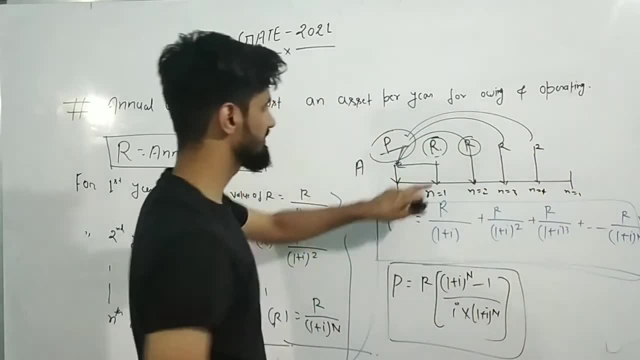 to 3. year at n is equal to 4. year at n is equal to 1 year. Each and every year you are getting a cash flow in the project p? r. then you are going to convert this cash flow into its present value. 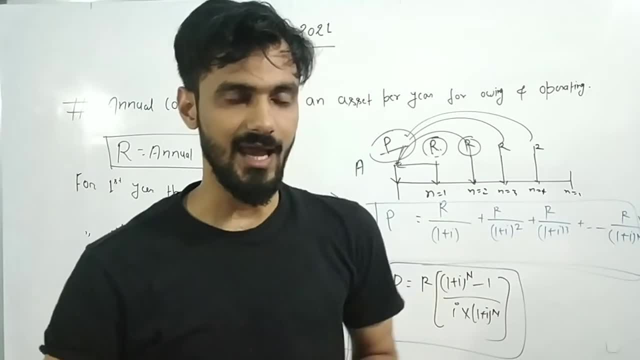 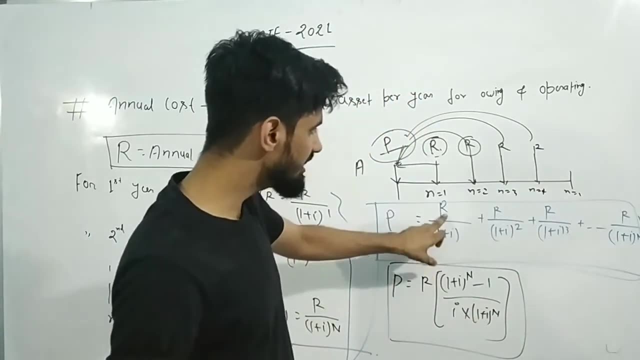 And after that you are going to convert this cash flow into its present value and after that it will be given with the sum of all of the present values and its cost in unit. then it will give you the original cost or the present value of all the assets. 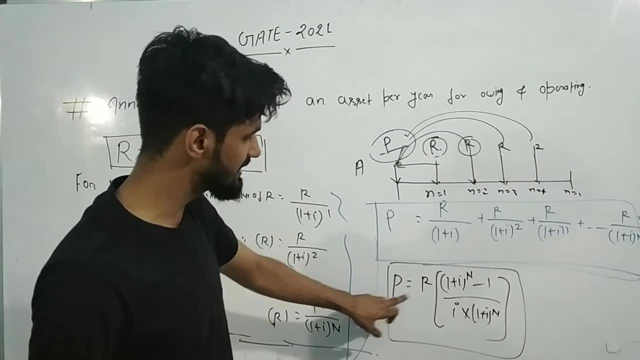 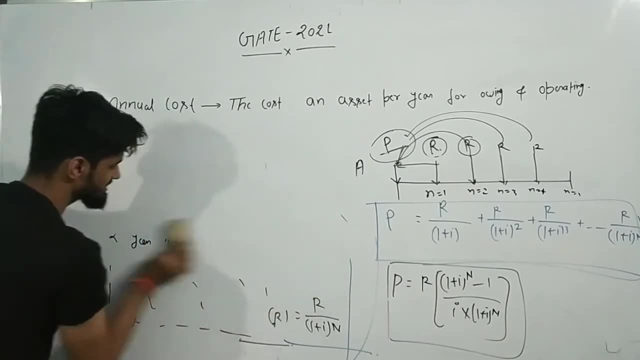 So its cost will be given for this total INSutta value. If present value is given, then you can calculate the value of r. So somewhere you can see this formula can be written in this way. I am just going to derive this formula in some other way. 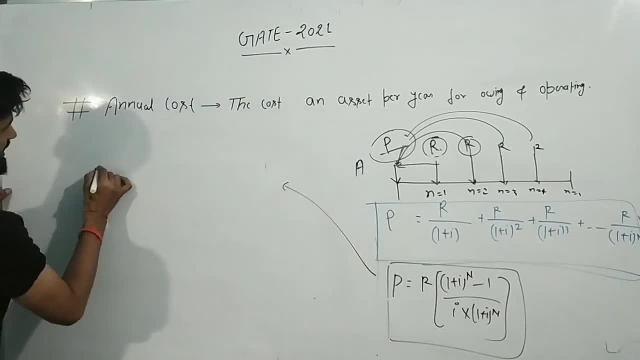 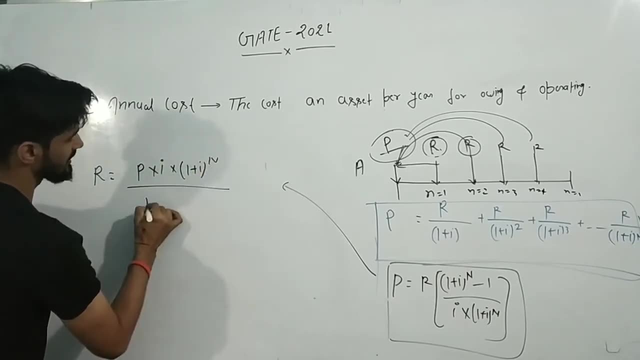 This formula can be written in this way also. That's why r is equal to p multiplied with i. I multiplied with 1 plus I whole to the power n upon 1 plus I whole to the power n minus 1.. Now if you will divide 1 plus I on the numerator to denominator, then you will get 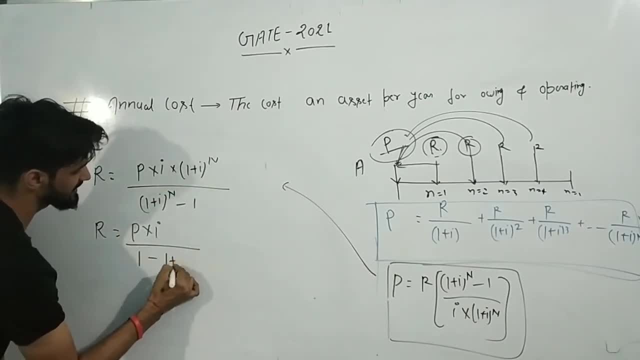 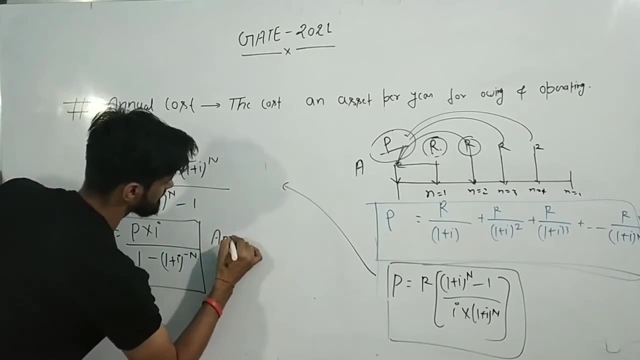 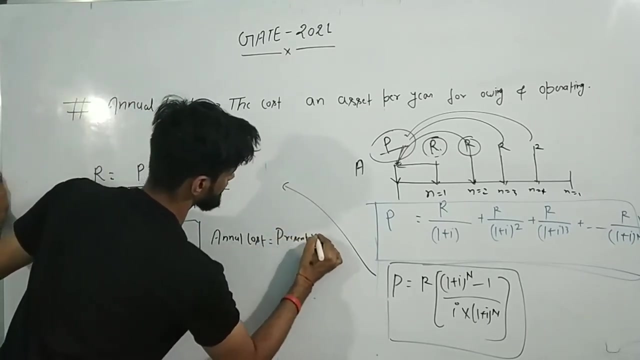 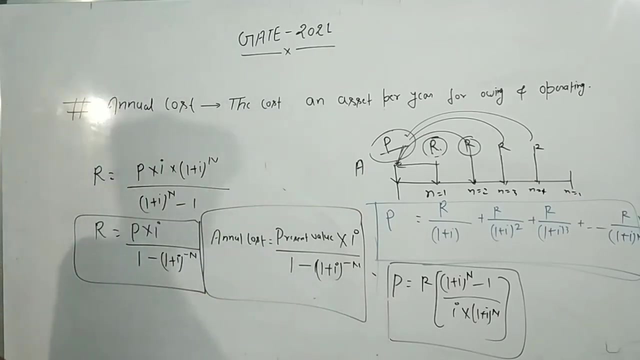 T into I upon what? 1 minus 1 plus I whole to the power minus n. So you can write annual cost. Annual cost is supposed to present value multiplied with rate of interest upon 1 minus 1 plus I whole to the power minus n. So sometimes error It can be asked in the form of formula. 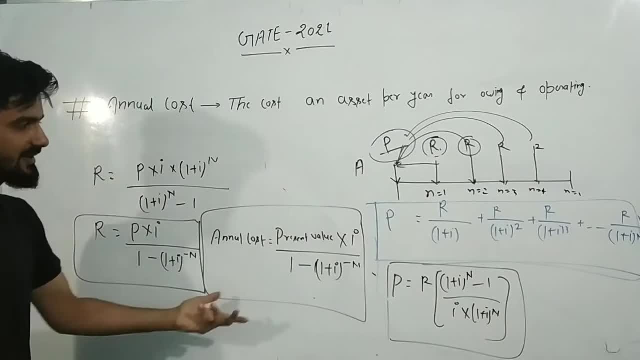 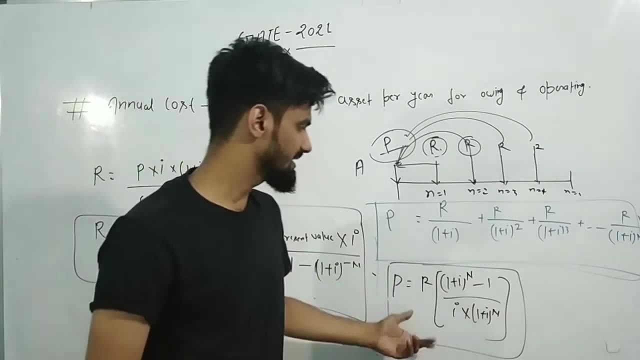 in the multiple choice question, Just like this value will be given or this value will be given, They will be asking about what will be the annual cost of the estimate. So you can calculate the assets if present value is B, Or in the numerical if they are giving. 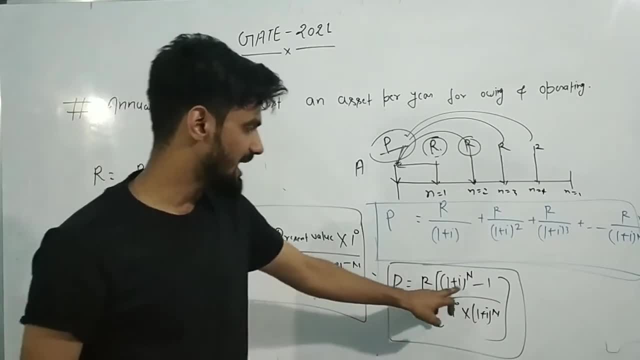 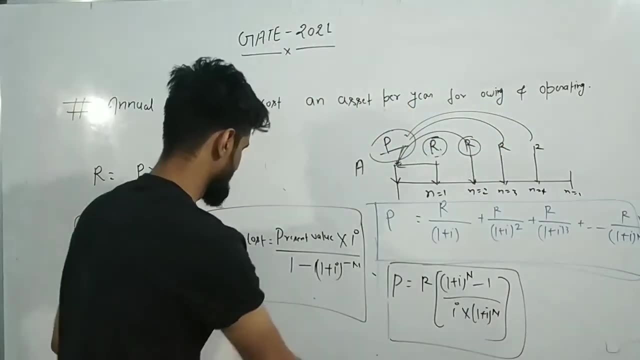 the present value is something: amount, particular amount, rate of interest will be given, service life of that asset will be given. then you can calculate the annual cost of that asset for the particular year. So now I am going to teach you. So what basically we are doing. 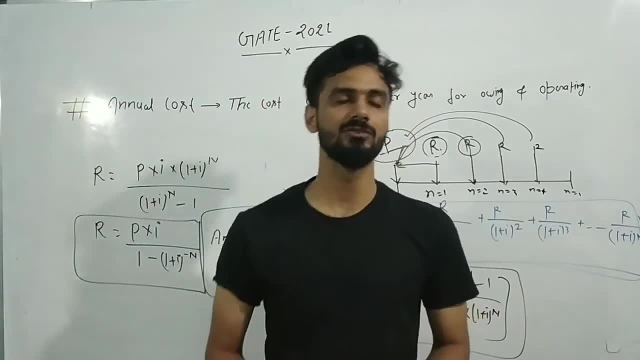 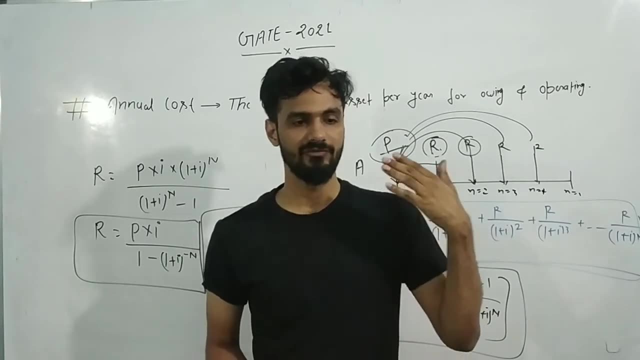 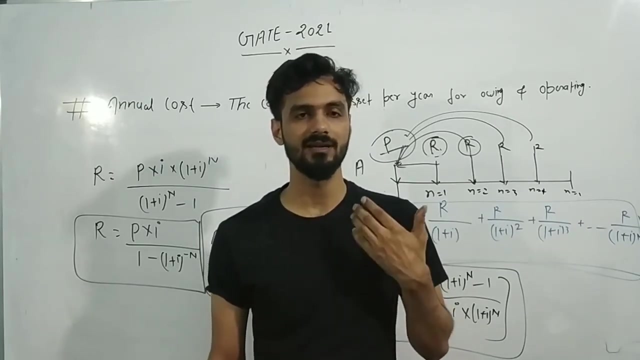 in annualized cost. In annualized cost generally, we are going to do only qualitative calculation. We are going to, you know, fix a qualitative calculation with the help of quantitative judgment. We are going to do nothing in the annualized cost Generally. we are just putting or we are just going to. 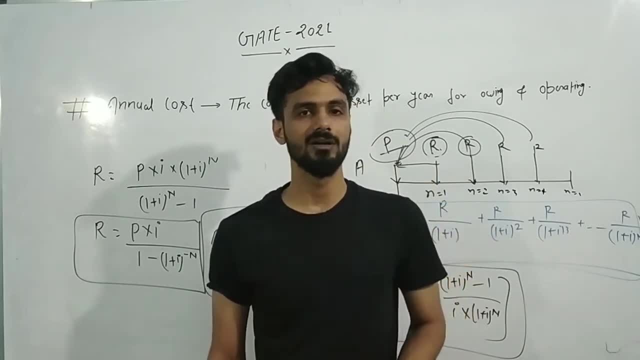 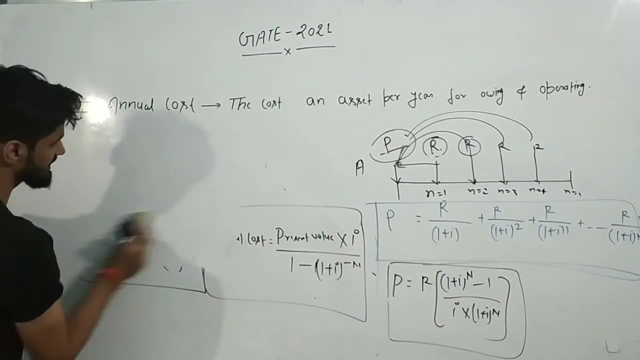 set a qualitative calculation on the basis of quantitative calculation, on the basis of a qualitative judgment and nothing else. Okay, Understand with the help of an example. I am letting you understand with a by good example, then you will be able to understand. 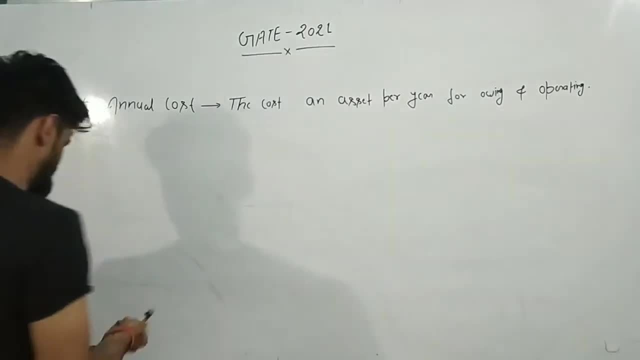 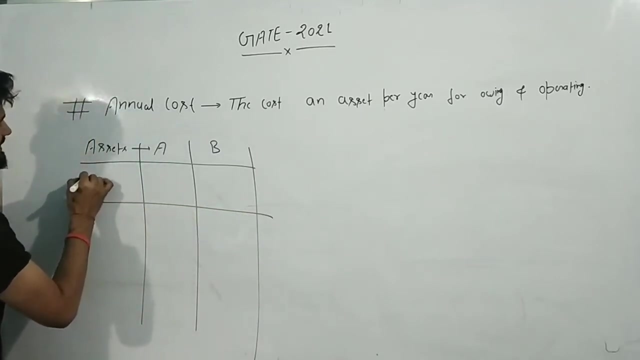 how we can calculate the annualized cost for that particular asset Assets, Just like I am just taking two assets, Asset A and asset B. Okay, Asset A and asset B. For asset A, present original cost. I am writing: Original cost for this asset is equals. 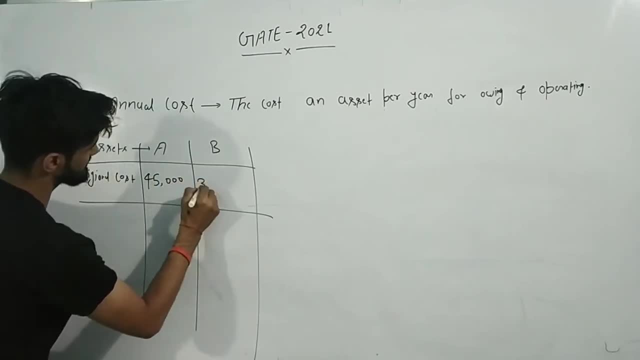 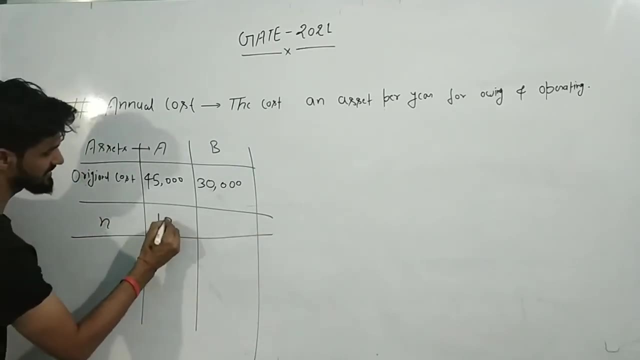 to 45000, for the asset B is equals to 30,000.. Okay, Now the service life, and that is equals to: for this is 10 years. for this is 10 years Now, operating cost is equals to 8000 and year. 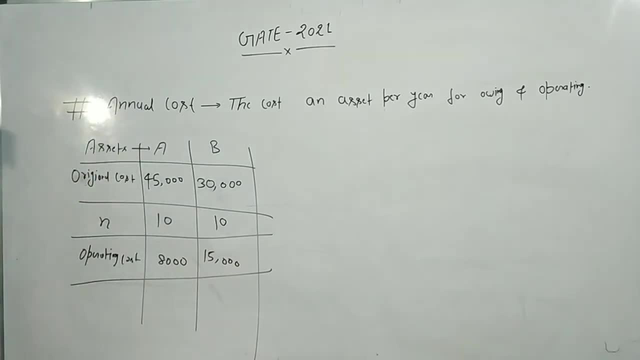 it is a 50,000.. Okay, 50,000.. Now here the rate of interest. rate of interest that is equals to year is 10%, and year is 10%. okay, So already I have defined you Here this. 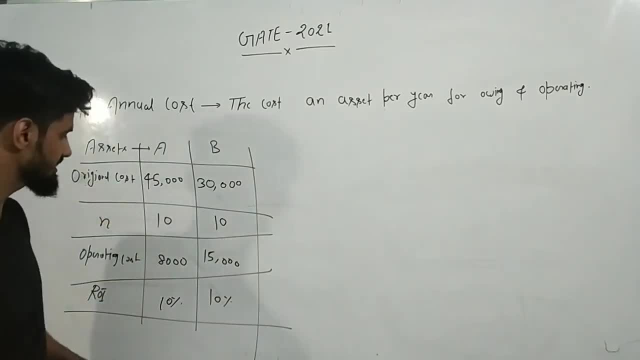 is the rate of interest. You can understand: here operating cost is given 10,000 and here operating cost is given 18,000 and it is annual operating cost. I am writing If annual operating cost, generally operating cost, will be given in the annualized form. 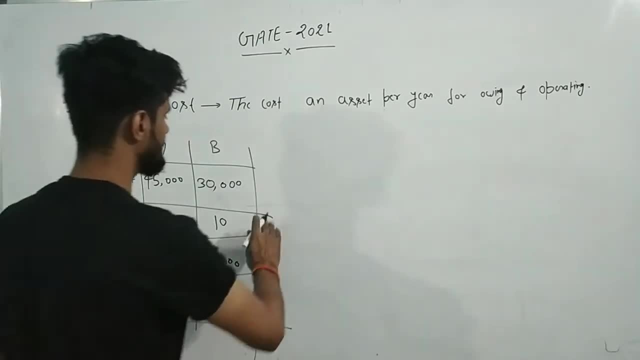 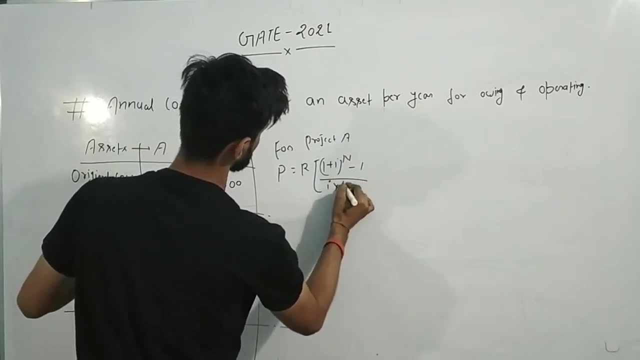 Now, how will you calculate these things? Just a suggestion: if you want to calculate first project A, So you can write formulan: p equals to R1, 1 plus i. whole-tex power 1 minus 1 upon i into 1 plus i. whole-tex power n. 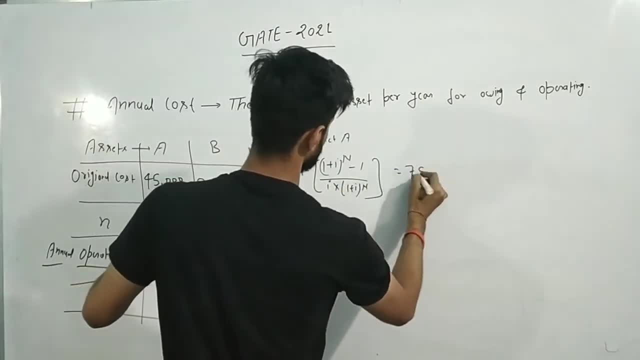 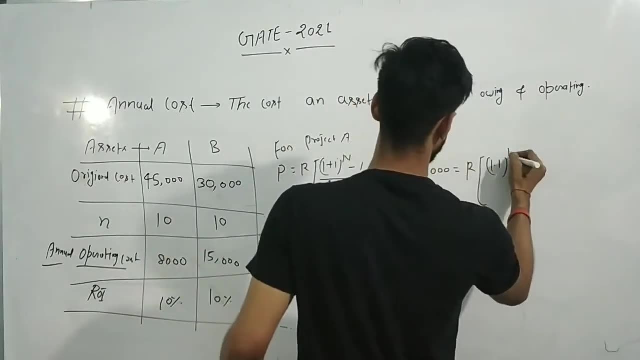 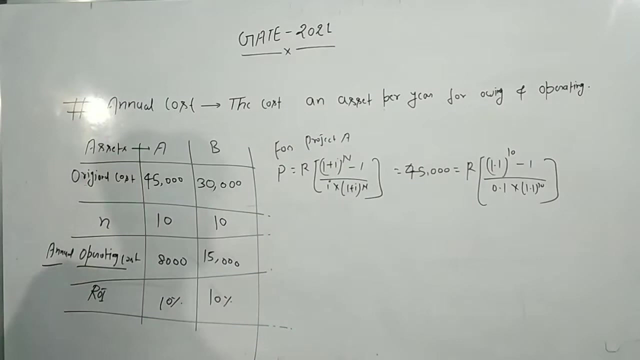 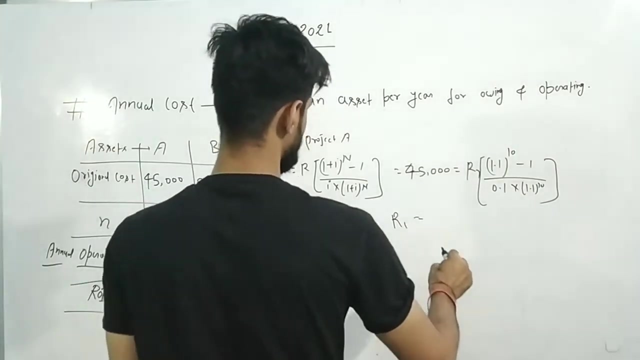 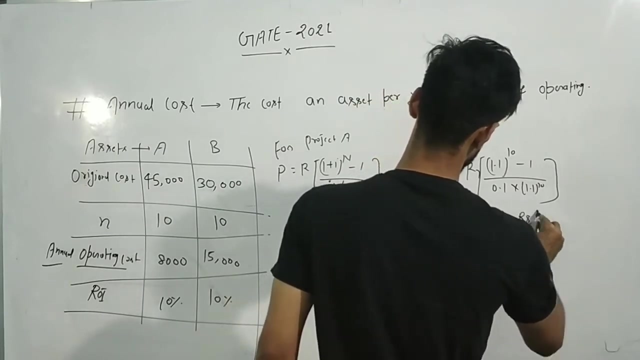 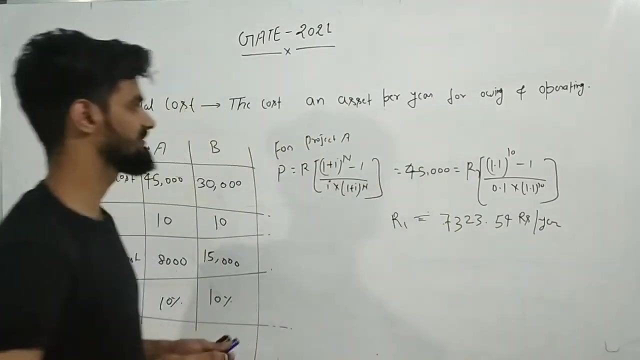 So here you can calculate R- that is supposed to be R- into one point 1 as whole-tex power: 10 minus 1 upon zero point 1 multiplied with 1 people power, 1 point 1. So from here, if you will see, then you can get the value of here I am writing- is R1, R1, R1, that is equals to 7323.54 rupees per year. you can write it in 7323.54 rupees per year. 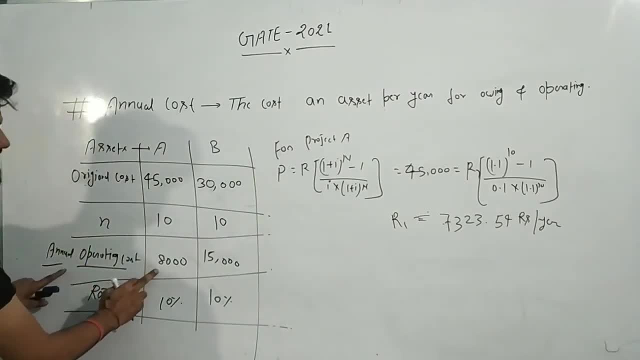 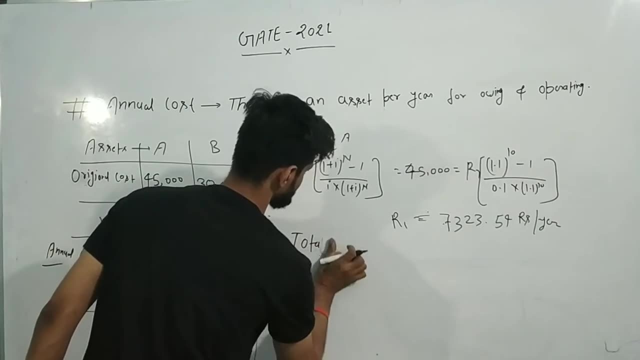 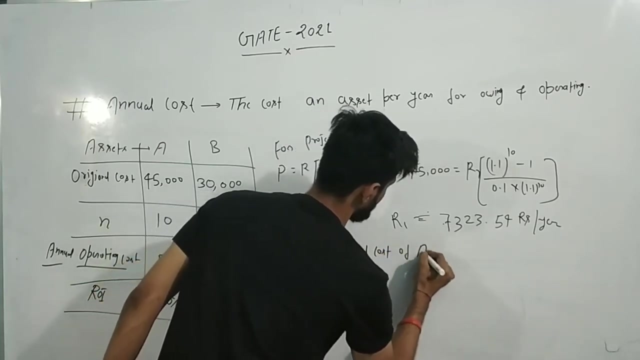 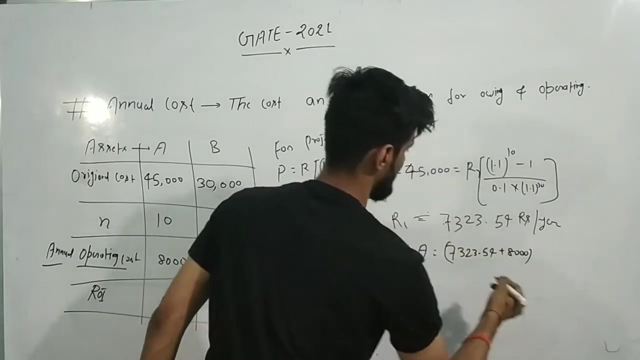 Now, if you want to calculate, this is operating cost. okay, so total total annual cost of A that is equals to how much? 7323.54 plus 8000, if you will add it, then you will be getting 5323.54. 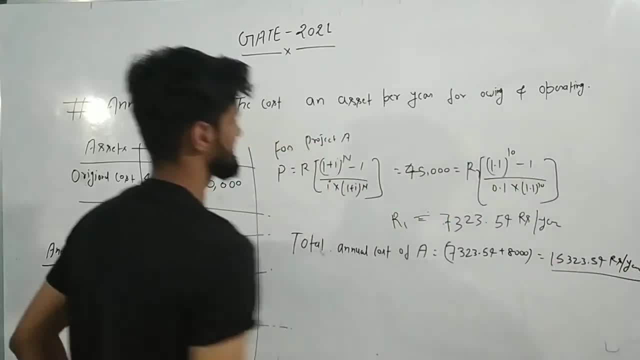 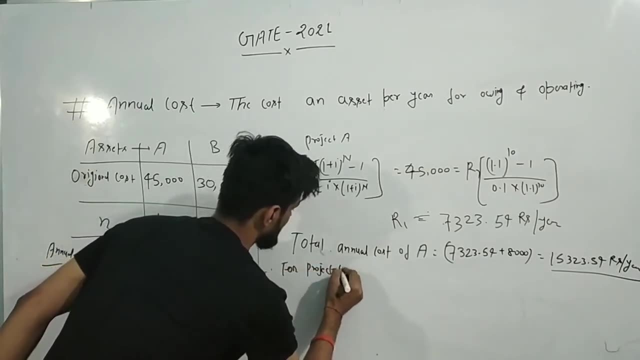 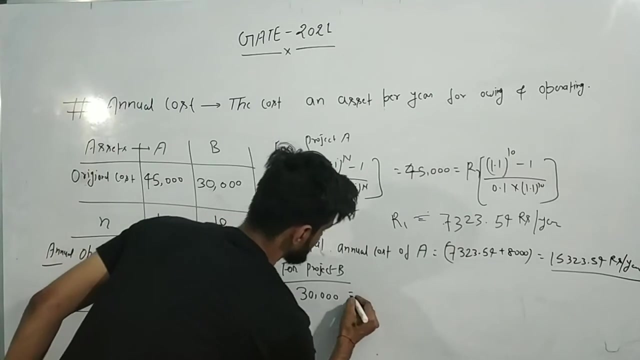 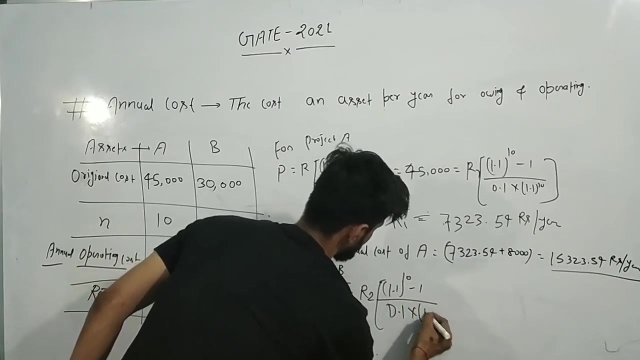 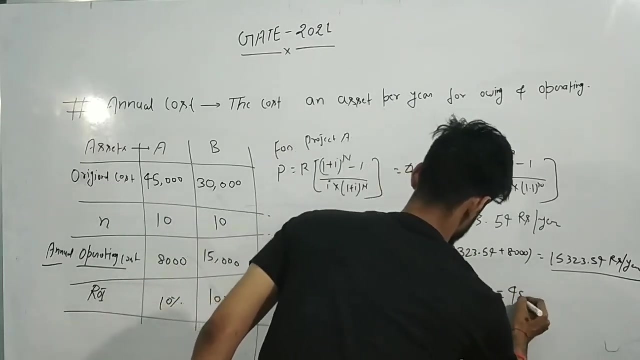 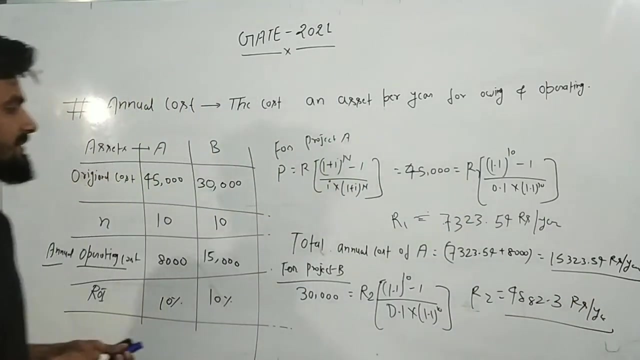 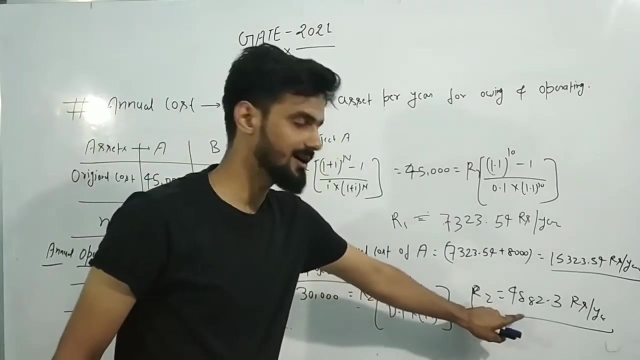 Rupies per year. that much amount. So you are getting. R2 equals to 488.2.3 rupees per year. Here it is, the. here R2 is what The value of R2, that is equals to what Each and every year, the you are going to convert this 30,000 rupees into annual cost and that is it okay. 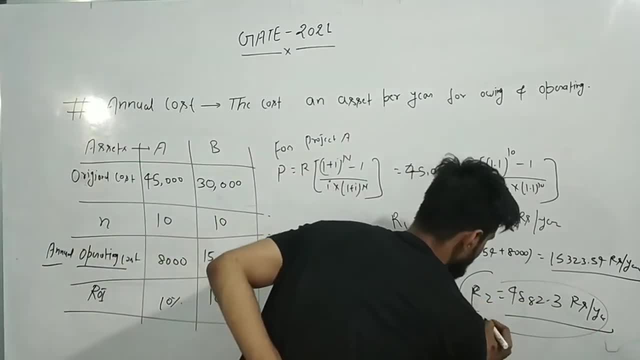 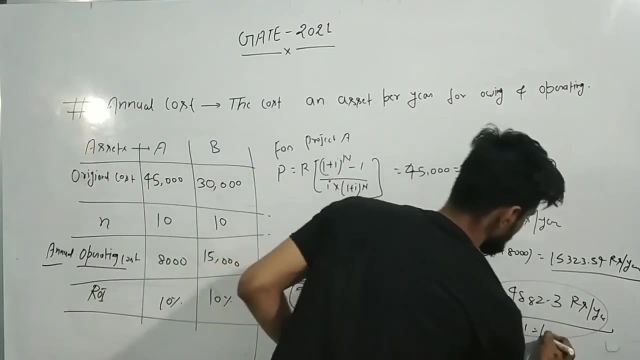 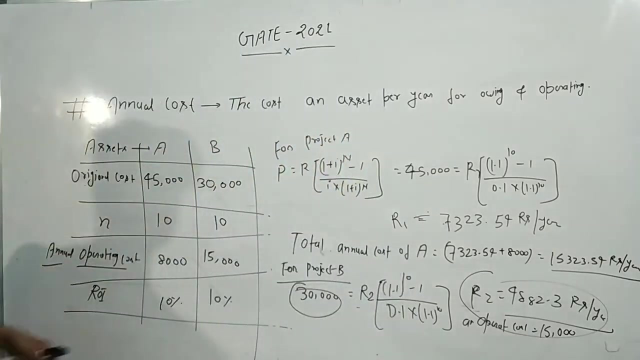 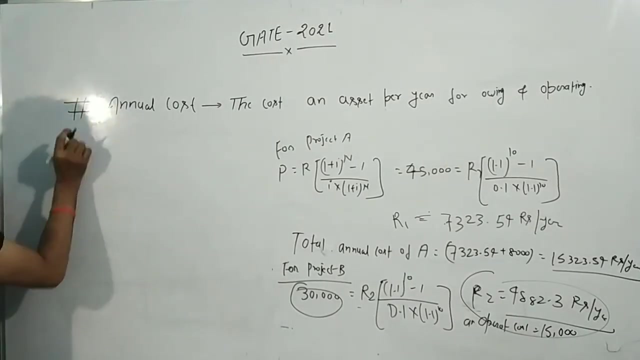 Now the operating cost for this is here. annual operating cost that is given in the question. that is equals to 5323.54.. So if you want to write then you can write. I am just roughing it out. so if you from here you can calculate total total annual cost of project B. that is equals to how much? 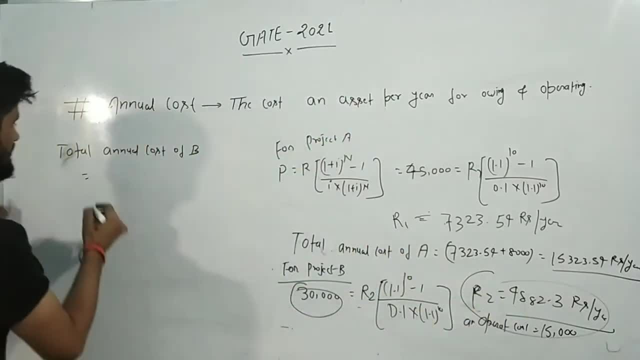 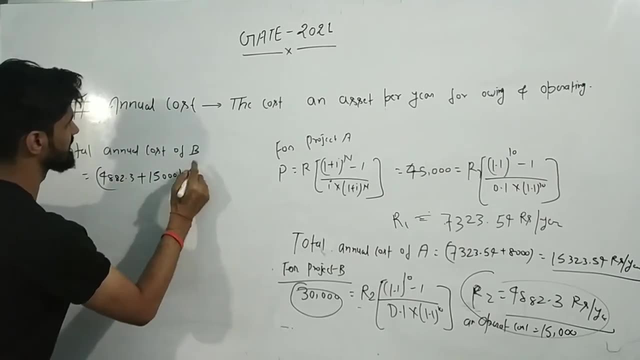 So here you have got the 488.2.3 rupees 488.2.3.. So here you have got the 488.2.3 rupees 488.2.3.. So here you have got the 488.2.3 plus 15,000 rupees per year. 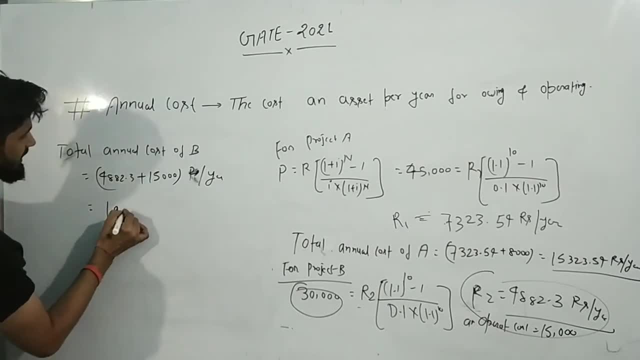 So, after calculation, you will be getting 1982.3 rupees per year. So, my dear friend, if you will see annual operating cost, AOC of A, that was equals to how much amount of rupees? 15,323.5 rupees per year. 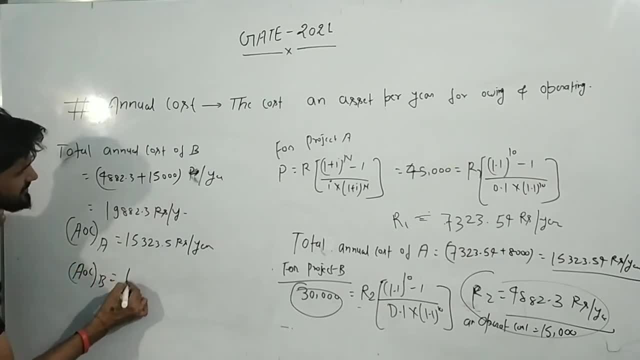 15,323.5 rupees per year. So, my dear friend, if you will see annual operating cost of B, that is equals to then on to 1988.2.3 rupees per year. Now what you have to do, just you are going to select the attractive project on the basis of annual cost. 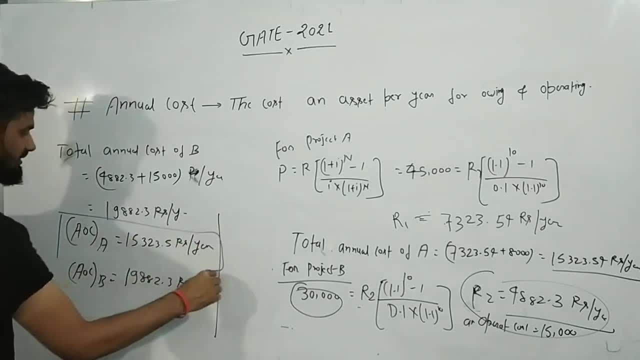 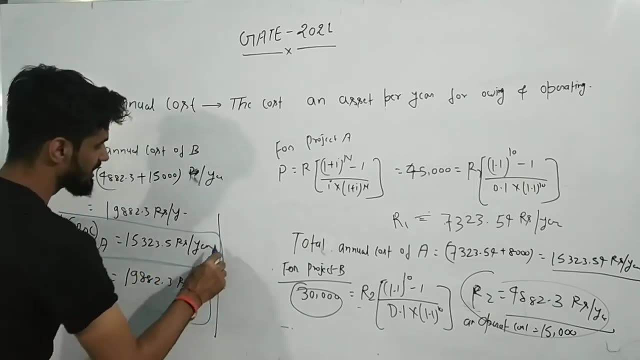 So here you will see the annual operating cost of annual cost. total annual cost of project A is 15,000 and total annual cost of project B is 19,000.. So the annual operating annual cost of I am writing here is only annual cost, okay. 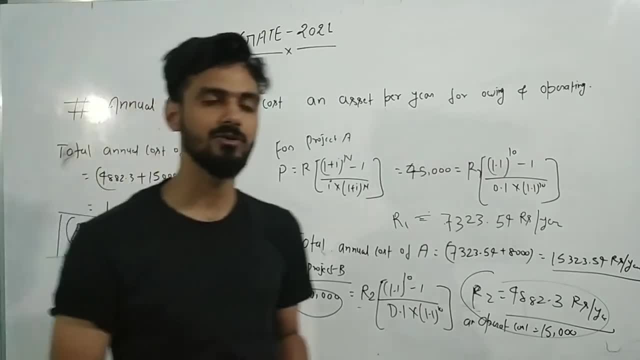 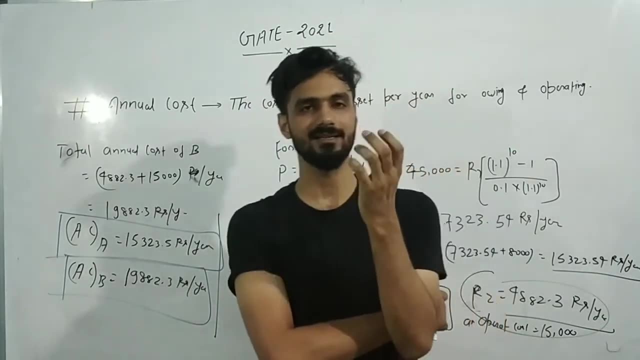 On annual cost of project A is less than as compared to annual cost of project B. So our you know if the annual cost of project we will be get more attractive to our goal product which are having less annual cost as compared to the project which will be having more annual cost. 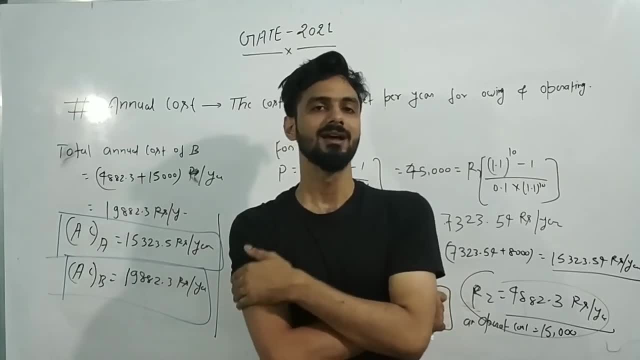 So here in this example you can see the project A is having less amount of annual cost than as compared to the project B. So our project is so project A will be more attractive as compared to project B. So so we have, we will. 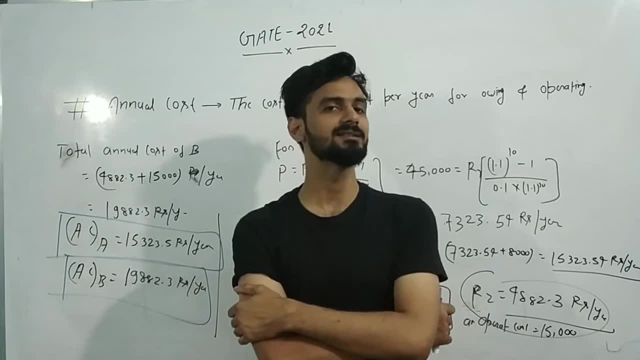 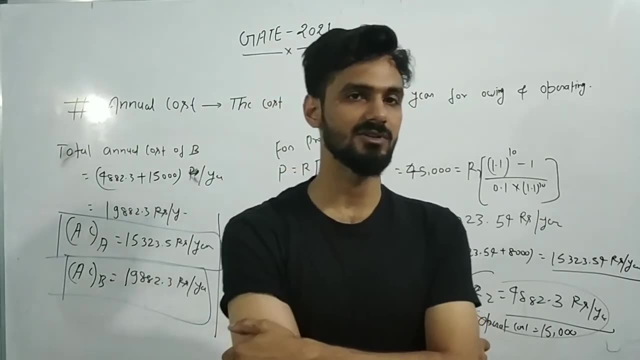 We will be more interested in investing our capital in project A as compared to the project B. okay, So this was the topics that I have taught here right now, on the basis of annualized cost, Each and everything I think, up to this year. you all have understood this. 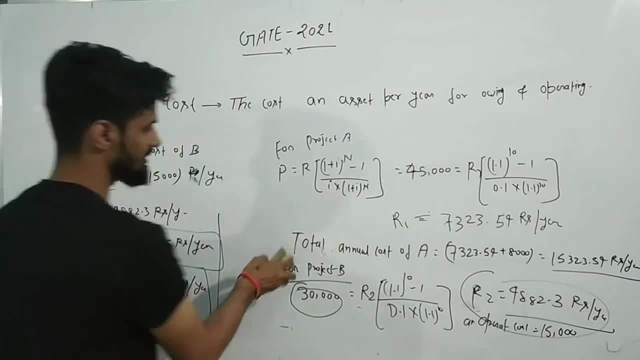 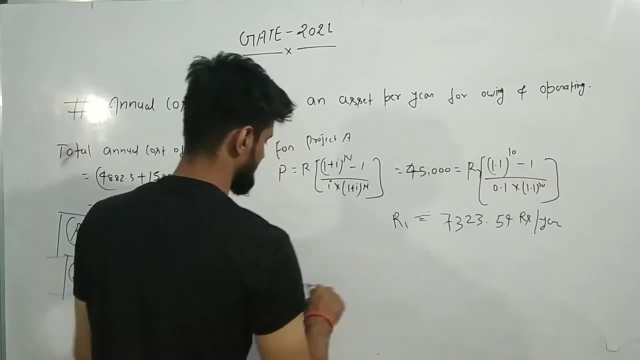 Now understand what is this thing? 7330, I am just letting you to understand with a of a cash flow diagram. Then it will be very clear to all of you For project A, what is happening here. if you will see, here the N is supposed to like: 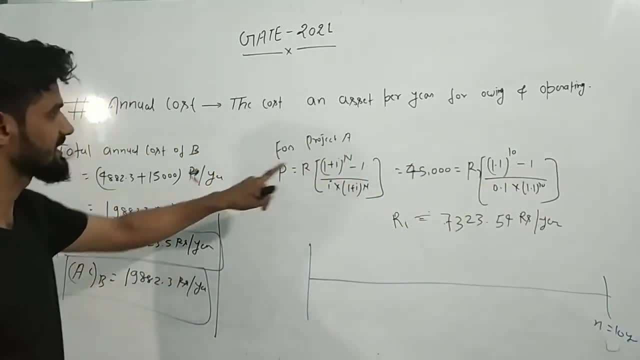 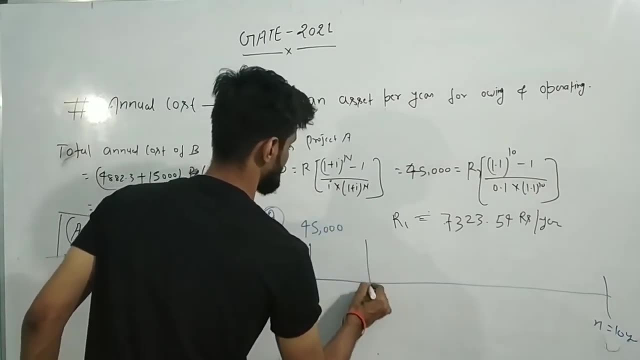 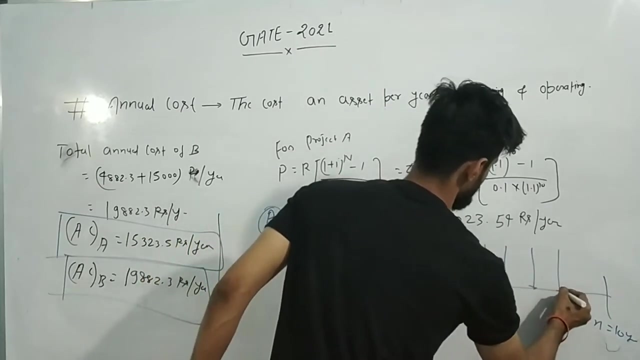 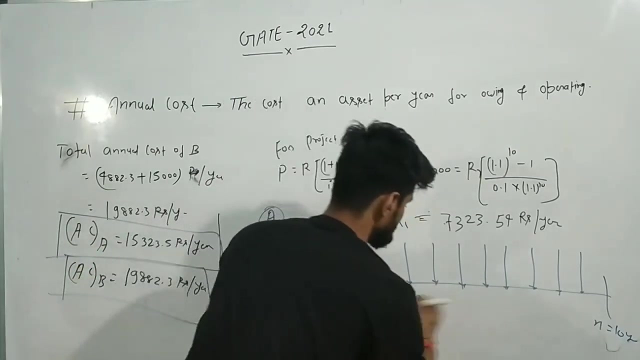 like service life is 10 years. here you are going to invest an amount of how much rupees For project A. I am writing: you are going to invest an amount of 45000 rupees. Now, here you are writing, each and every year: okay, at N is equals to 1, N is equals to 2,. at N is equals to 3, N is equals to 4, N is equals to 5, N is equals to 6, and so on. 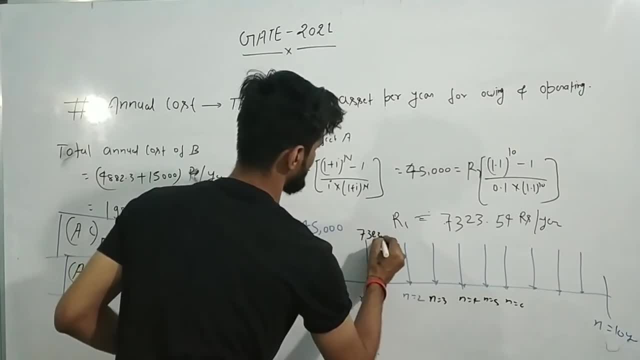 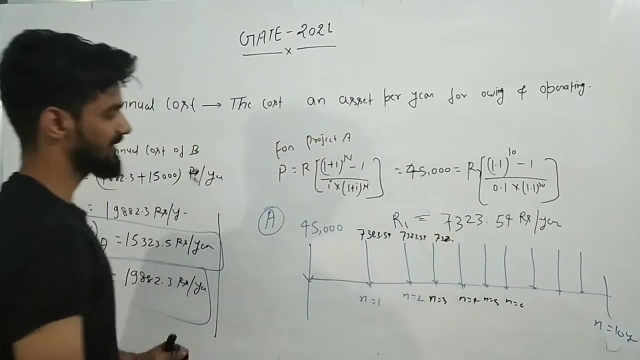 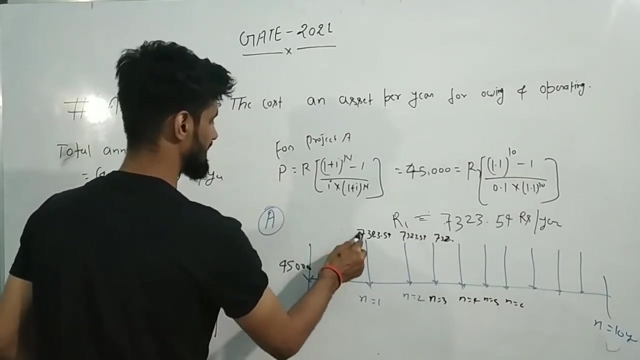 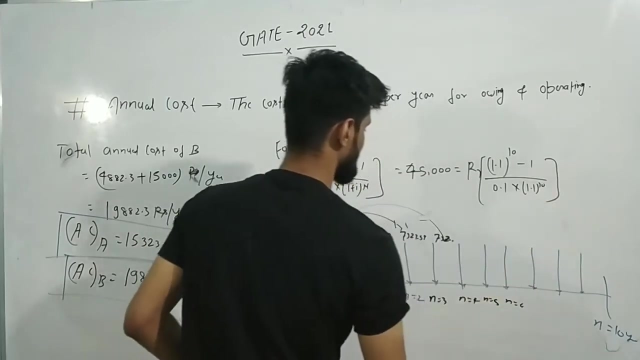 and so on. you will be getting here how much amount: 7323.54,, again 7323.54,, 7323.54,. so now what is happening here? if you will be converting- just rough it out, here I am writing 45,000, if you will be converting it, all these amount, into the annualized cost, if you will be converting all these amount in its present value, okay, in its present value. 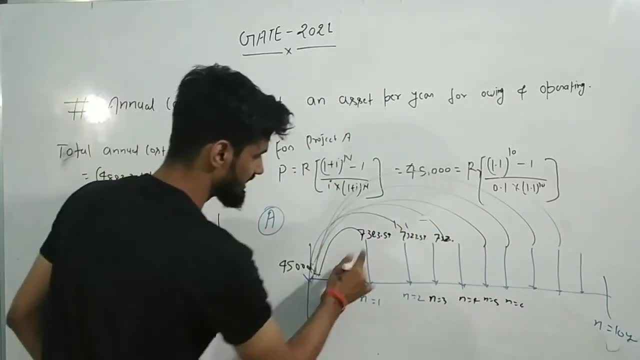 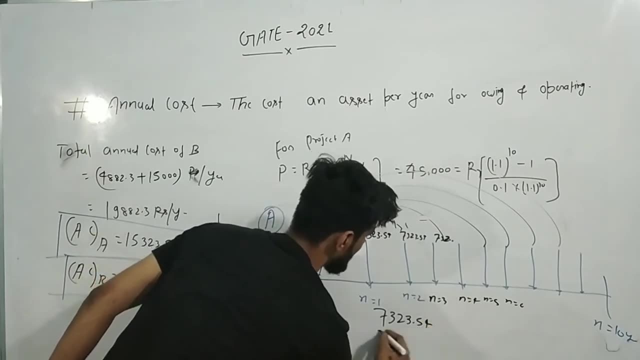 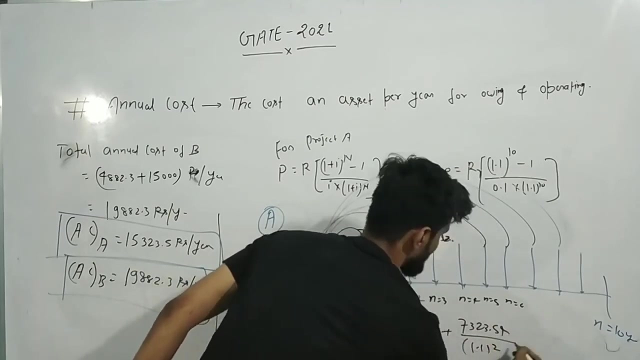 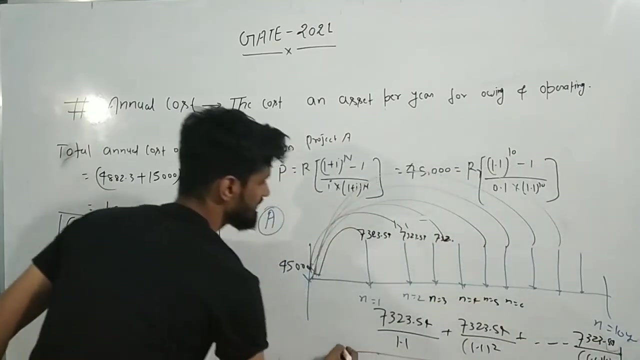 after calculation of present value, then how much amount of you will be getting. if you will just calculate- so here I am just converting it into the present value- then again you will be getting 7323.54 upon 1.1 plus 7323.54 upon 1.1 bullet square, plus 7323.54 upon 1.1 bullet square 10,. so now, if you will add all these things, all these value, because already I told you, if you are going to convert all the cash, 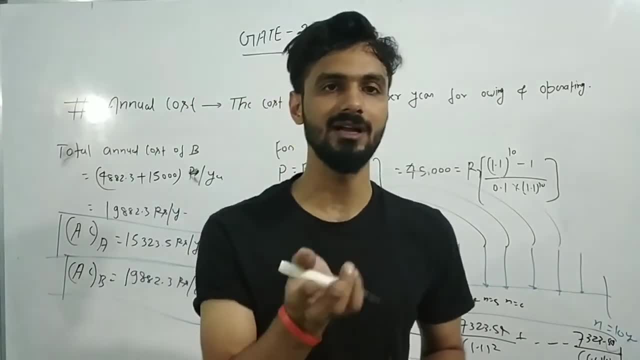 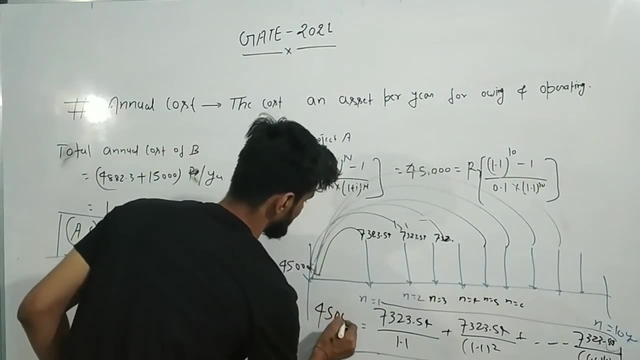 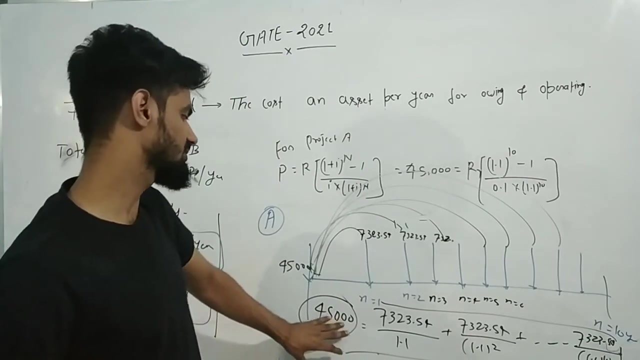 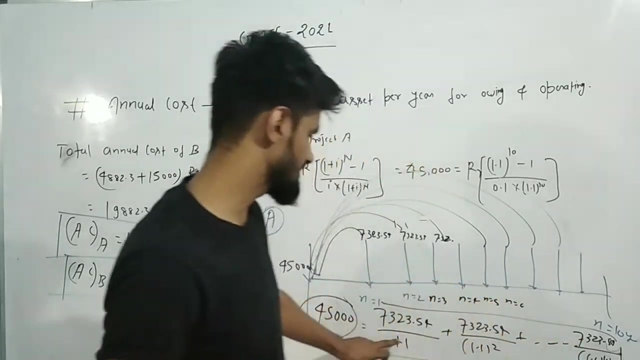 flow in its present value, then the sum of all these cash flow will give you the net original value of that asset. so you will get 45,000 from here. you will be getting 45,000 here. if you are getting 45,000 from this particular value, then your answer is correct. but if you are not getting 45,000 after calculation of this value, then your answer will be wrong. so you can say your answer while calculation of this thing also and how it has come. already I will how this particular has come. we are doing this thing. 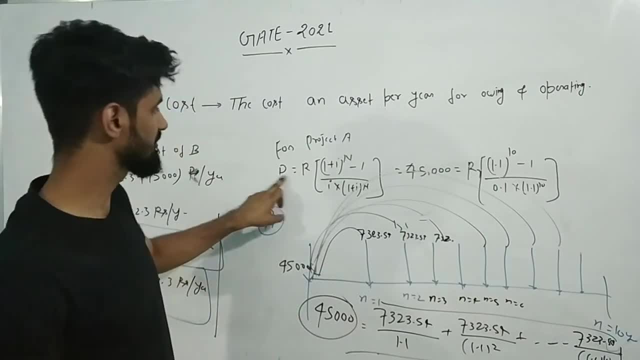 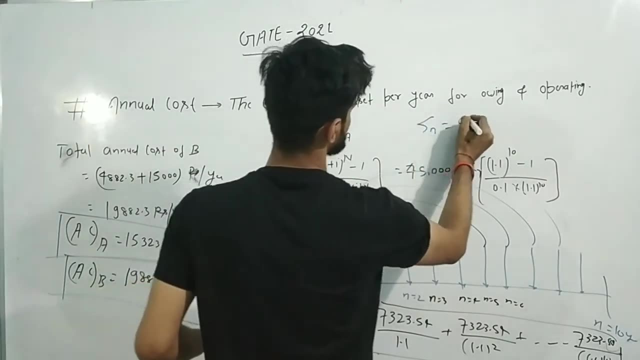 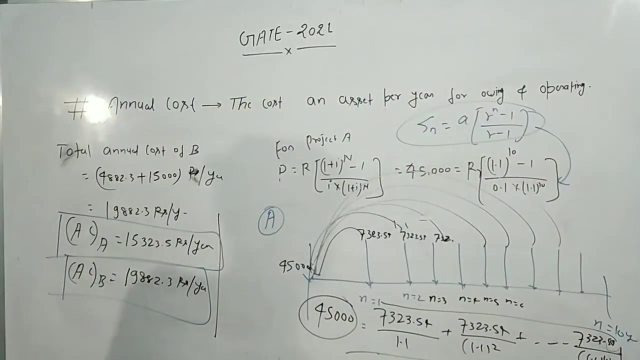 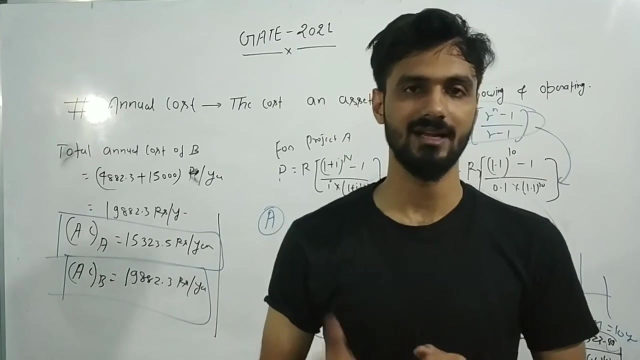 only okay, already from here, you can go from here because it will be a gp term and already you all know the sum of gp, as in is equal to, you can write: sum of gp is equal to a r equal n minus 1 upon r minus 1, that is the same thing I am doing right now in this particular. only okay, so you can do these things for project b also. so the same thing will happen, okay. so my idea is just practice this question. it is one of the good question that I have shown you right now on the board. in the next lecture I will be solving some different numeric. 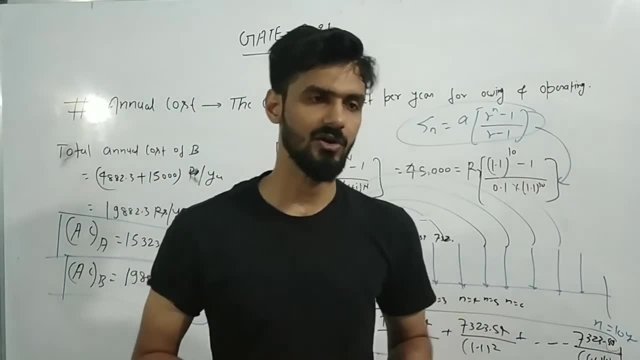 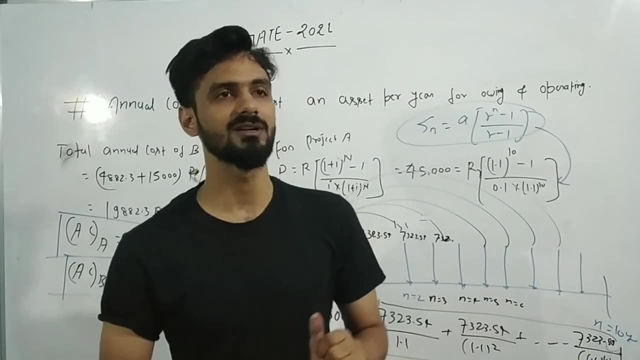 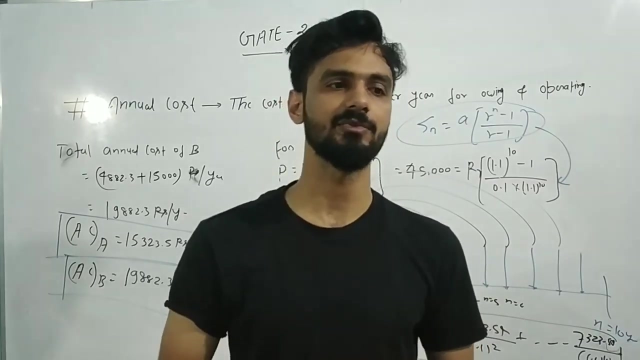 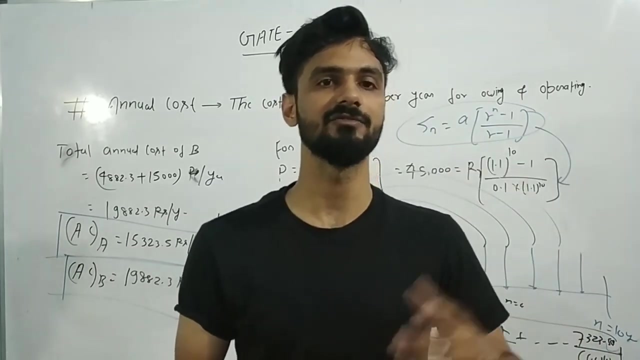 details. that gate has not asked up to this. okay, on the basis of permanent, you know, permanent investment. already up to this time, gate has not asked the question. on the basis of permanent investment, if you are going to, you know, invest some amount of money in a project and in the question they are asking what we are investing 10,000 rupees for the permanent setup, for the permanent infrastructure building. these types of questions. gate has not asked up to this, so we will be, I will be. 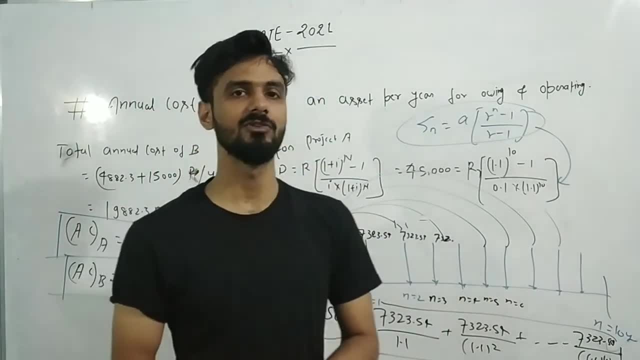 discussing in the next lecture that types of question. okay, so thank you for this lecture. okay, bye.